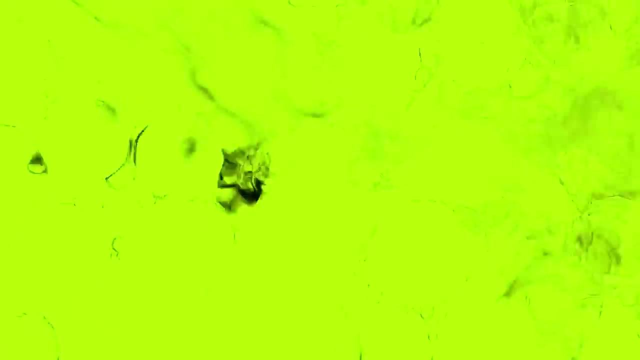 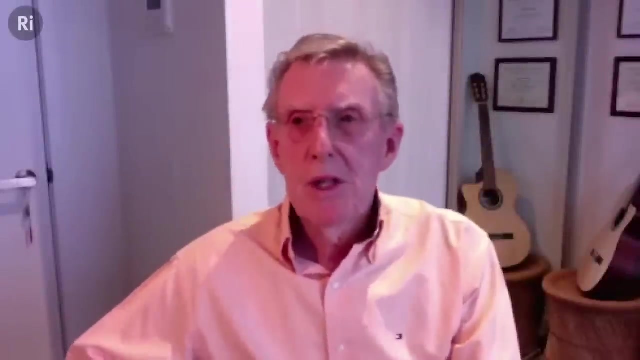 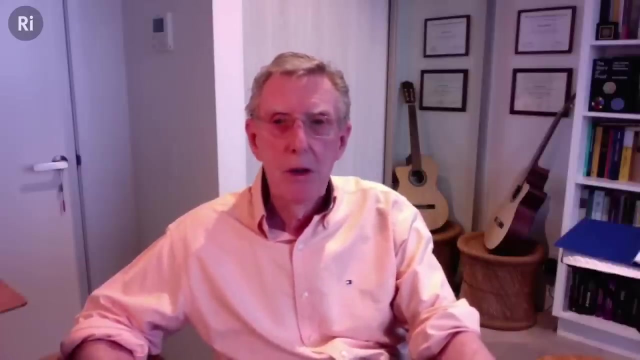 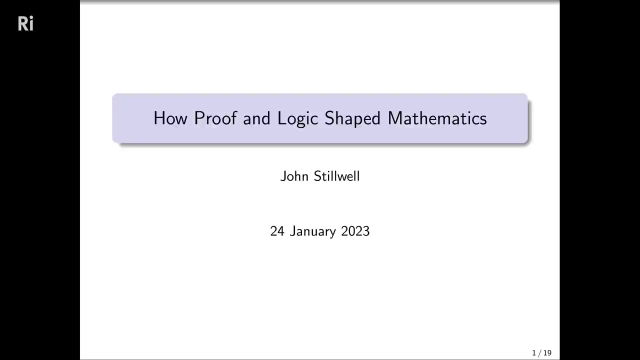 Well, thank you, Lisa, and thank you to all the viewers who've tuned in. I'd also like to thank Princeton University Press and the Royal Institution for giving me this opportunity to talk about my book. Now, why am I so obsessed with the idea of proof in mathematics? 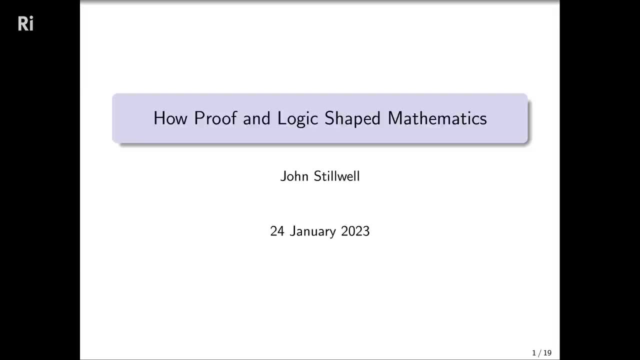 Well, one reason is that I think it doesn't get enough recognition in our teaching. Everybody knows that mathematics is about calculation, but more so, if anything, it's about proof, And that's what I would like to emphasize. Not that I've got anything against calculation In 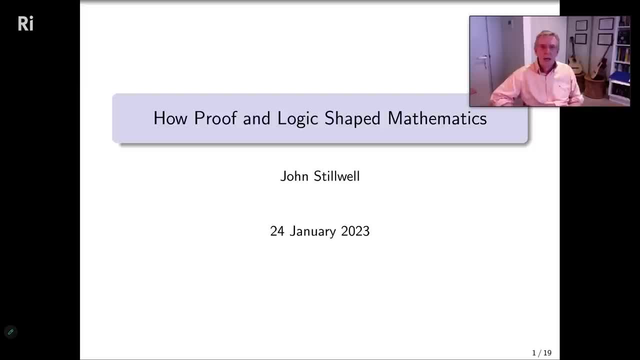 fact, one of the things I want to explain today is that calculation and proof are basically two sides of the same coin, But to see what I'm talking about, let's begin with the proof. Now, this is my favorite, and it's of the 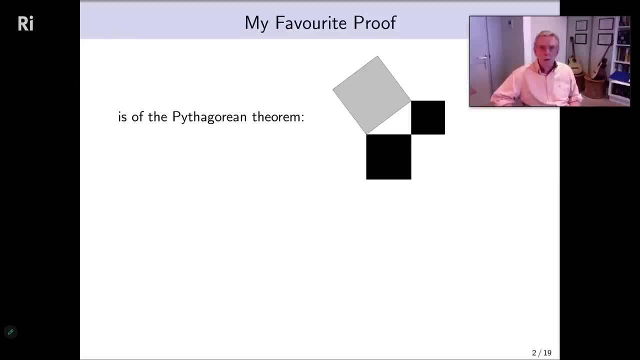 Pythagorean theorem which I'm sure all of you know- It's probably everybody's first theorem- and it says that the square on the hypotenuse of a right-angled triangle is equal to the sum of the squares on the other two sides. Now there's a lovely visual proof of this, probably a very 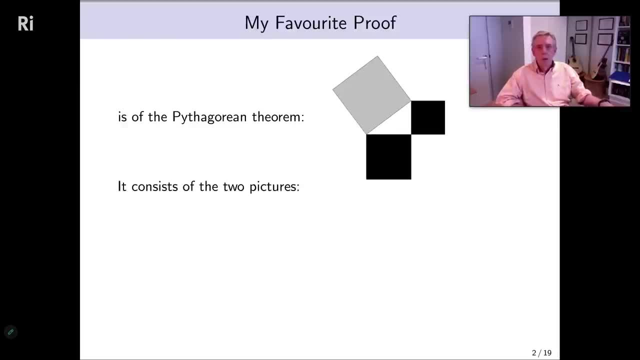 ancient proof, Even before Pythagoras possibly, And it consists just of two pictures. The first picture takes four copies of the triangle and arranges them in a square sort of head to tail like this, And it's clear when you do that that the remaining space is simply the. 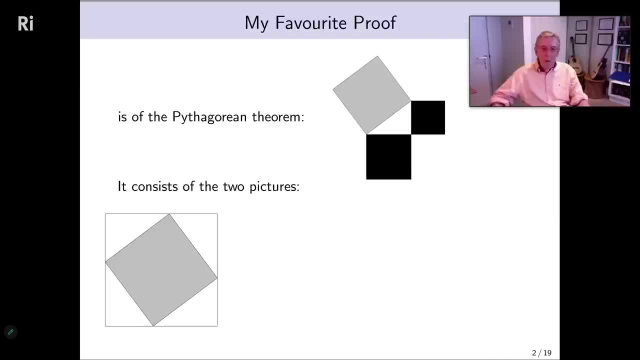 square, on the hypotenuse, the gray square. But if you rearrange the four triangles like this, the remaining space, The remaining space is obviously the squares on the other two sides, the black squares. Therefore, the gray area is equal to the black area, which is precisely Pythagoras' theorem. 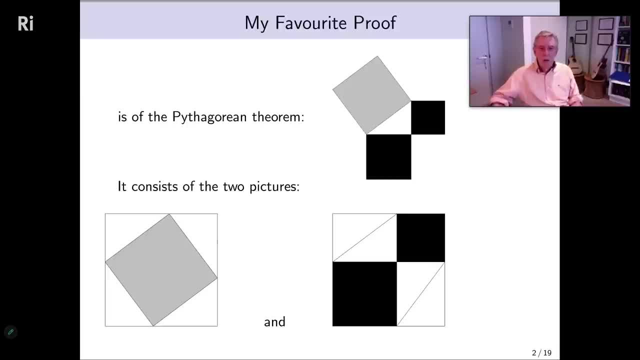 It's very clear, it's very simple and you see it immediately. In fact, I believe the word theorem means what is seen. That was the original meaning, But if you think a little more you might quibble slightly, Because we may have been deceived by these pictures. It's not absolutely certain that. 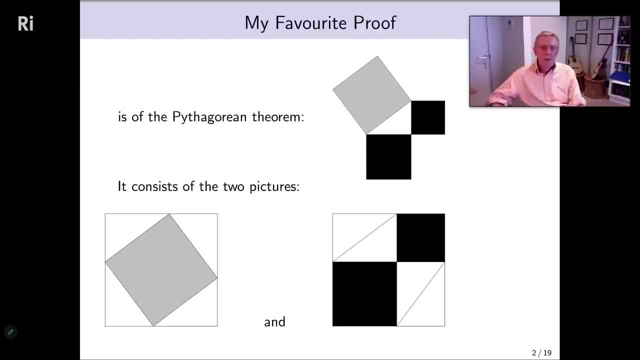 that gray area is square. You would have to check. I think that the angles in the corners are right angles. And if you look in Euclid, for instance, for his proof of the Pythagorean theorem, you'll see. it's entirely different from this. It starts with some very simple assumptions, like: 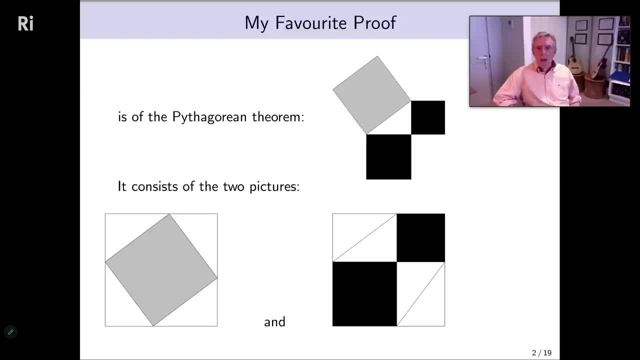 there's a line, so you only need two points And it proceeds to develop a theory of areas of rectangles and parallelograms and triangles, And then it carefully transforms the squares on two sides of the triangles to the square on the hypotenuse. So it's very convincing also, but also very elaborate. 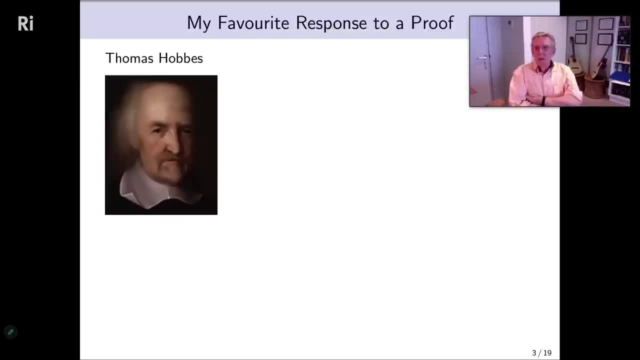 And this led to a remarkable reaction to Euclid's proof, which I enjoy immensely. And of course it's the reaction of Thomas Hobbes, the English 17th century philosopher, who apparently didn't meet geometry in his younger days. He first came across it when he was 40 years old. 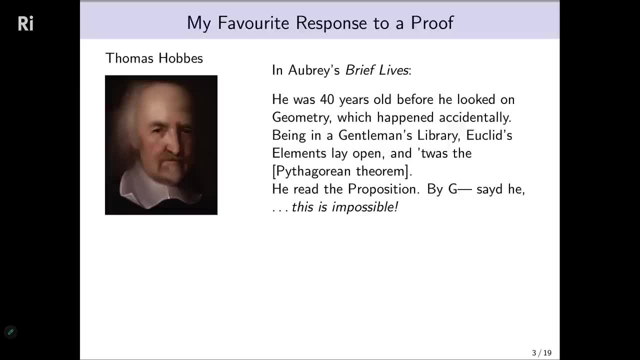 and happened to see a copy of Euclid's Elements in the Gentleman's Library And it was open to the Pythagorean theorem, which he read And he said: by God, this is impossible, And I don't blame him entirely If you hadn't seen that proof I just showed you. it does seem very surprising that. 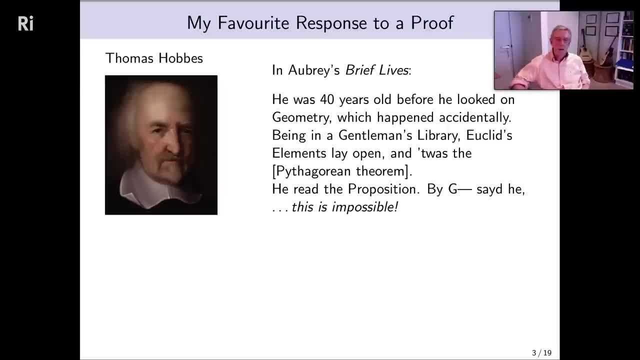 there's a simple relationship between the sides and the hypotenuse of the right angle triangle. Well, what did he do? He read the proof, which referred him back to some other proposition, which referred him back to another, that at last he was convinced of that truth. 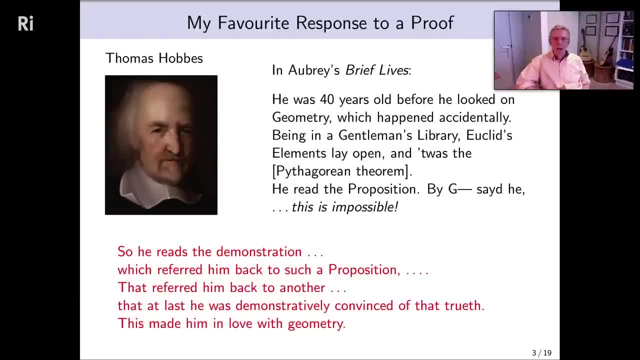 This made him in love with geometry. A wonderful story, And it also illustrates the way proofs work. You find simpler things on which the proof depends, and then simpler things on which they depend, And finally you get back to self-evident propositions, which are known as. 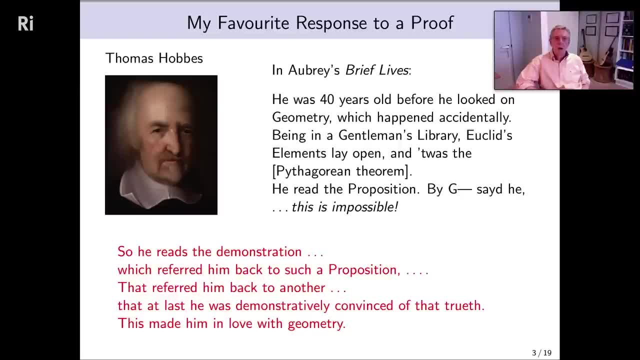 axioms. So that's what Hobbes was impressed by: the fact that this surprising theorem follows by logic from self-evident statements about points and lines. But still, as I say, it is a very elaborate proof. And why did the Greeks go to so much trouble to prove something? 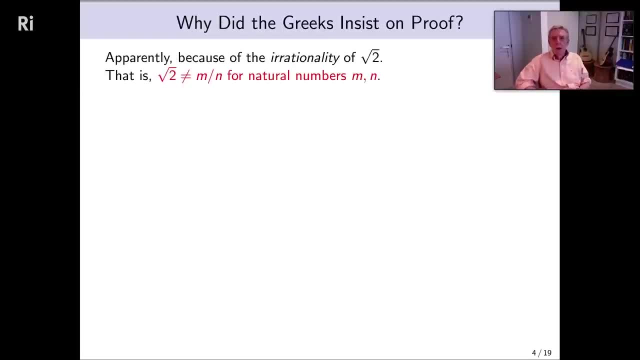 that you could just see. Well, it appears that the reason that they were so concerned about proof in geometry is another discovery of the Pythagoreans. And this is perhaps the more important discovery of the Pythagorean theorems, Because, as I said, Pythagoreans, as I said, Pythagorean theorem. 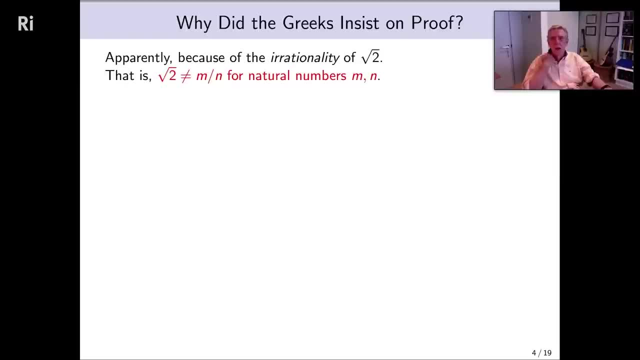 itself was discovered in many cultures, And that's why we're going to talk about the Pythagorean theorem, Because, as I said, Pythagorean theorems itself was discovered in many cultures, And this in India, China, Babylonia, before Pythagoras even. 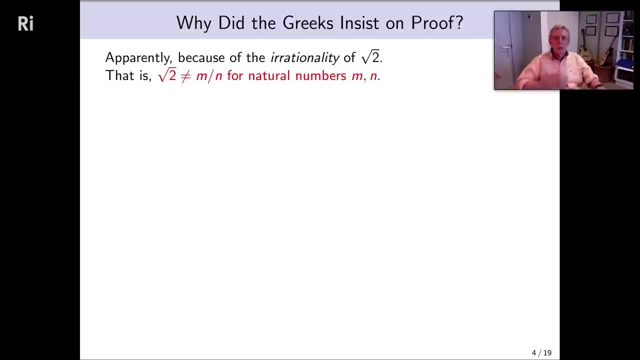 But what the Pythagoreans discovered, which was more influential than any of the other discoveries, is the irrationality of root two. Irrationality means root two is not a ratio of natural numbers. That's what irrationality originally meant, not a ratio. 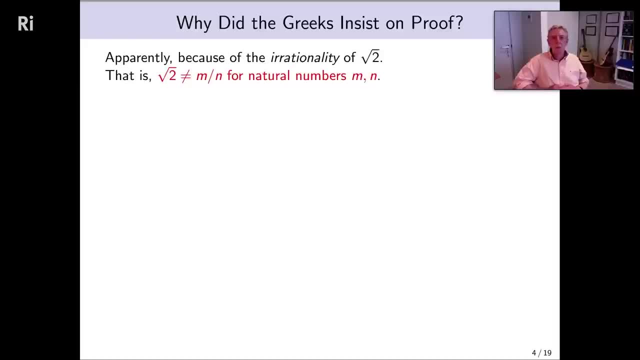 But of course it always seems to us to mean crazy or senseless. And this dual meaning is also what the Pythagoreans thought, because this very much upset their theory of the world. They believed, or hoped that everything could be explained in terms of whole numbers. 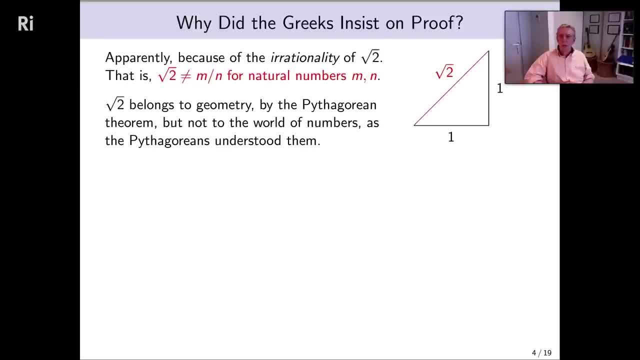 But by discovering root two is not explainable. in this way, they've discovered There's a kind of chasm between geometry and numbers, because root two certainly belongs to geometry- There it is as the diagonal of the unit square- But according to this discovery it doesn't belong to the world of numbers. 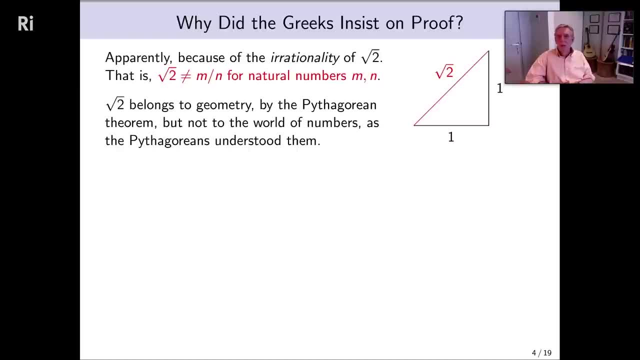 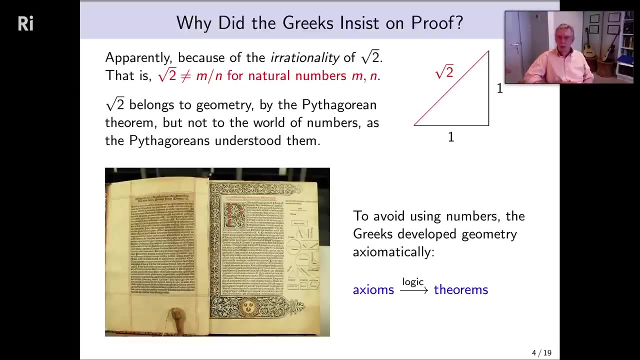 So there is a divorce between geometry and number theory, And they realized that to find the truths of geometry, they would have to take another approach, And that's the origin. And that's the origin of this axiomatic method which is exemplified by Europe. 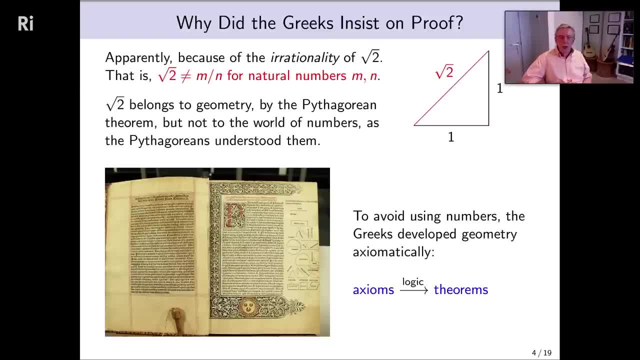 Here's a picture of the first printed edition of Euclid's Elements. But the essence of Euclid's Elements is that there are certain axioms, self-evident statements about points and lines and circles, and you derive theorems from them by logic. 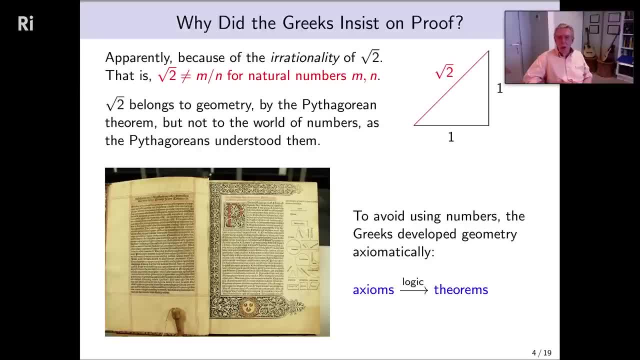 So everything follows in a, in an undeniable way, from undeniable statements. That's, that's the certainty that the Greeks were looking for in geometry. Now, that is the method that has survived the whole history of mathematics. Today, it's become the model of the way we develop mathematics. 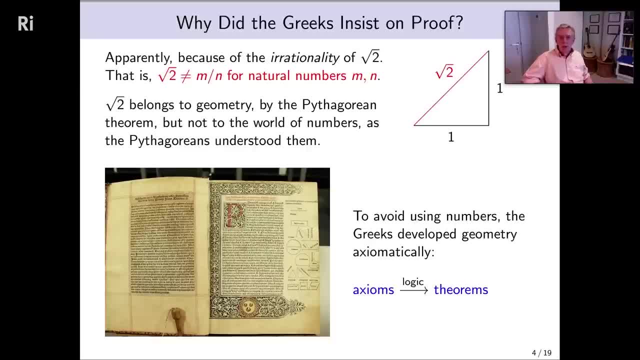 We take certain axioms, which might be self-evident statements or might be simply statements. you want to assume and and later find what, what things satisfy these statements. But in any case you have a starting point called axioms. 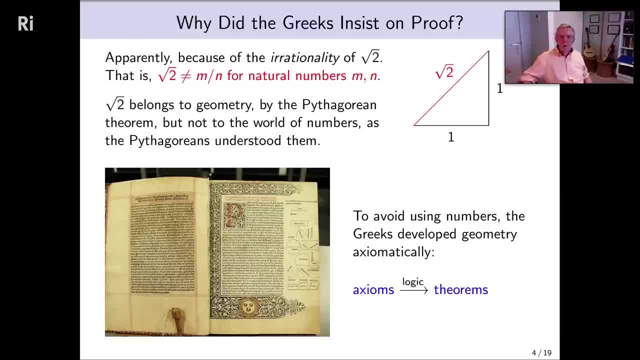 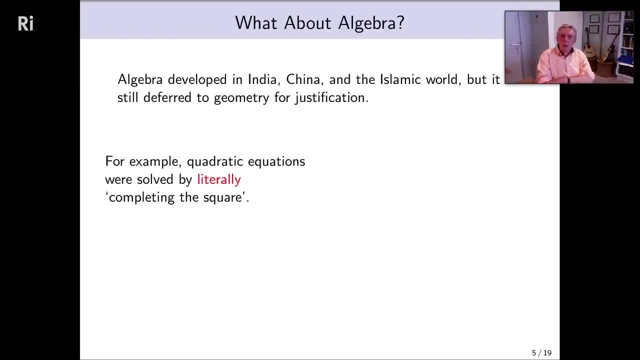 And by means of logic you deduce theorems. Now this sounds very different from algebra as we know it from high school, say. Algebra developed separately from Greek mathematics. In fact, the Greeks never quite got the idea of algebra. 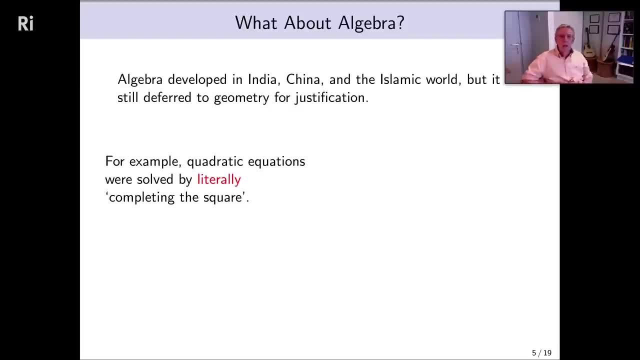 They missed. they missed something And algebra developed in India, China and the Islamic world, But surprisingly, it still deferred to geometry for justification. The example I want to talk about is quadratic equations. Now we talk about completing the square to solve quadratic equations. 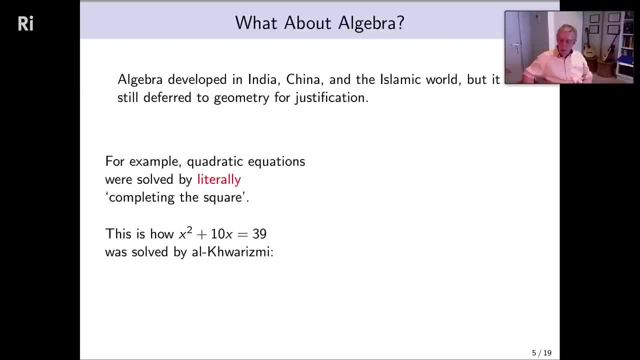 This was very literally what they did in the early days. I want to show you an example from Al-Khwarizmi, which is a is a book on algebra from around the 800 CE. Al-Khwarizmi was not the first to do this. 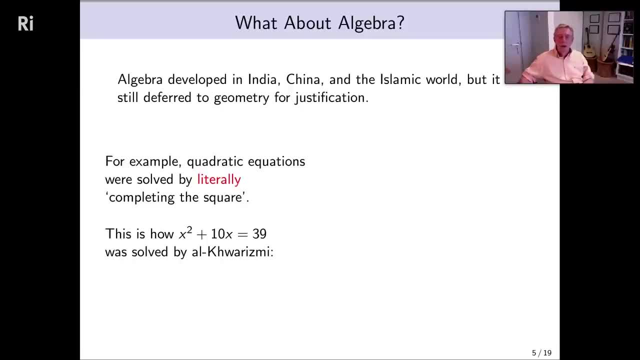 but he was the one who really made it caught. catch on Algebra as we know. it really begins with him. In fact, the name of his book gave us the word algebra, And his own name, Al-Khwarizmi, gave us the word algorithm. 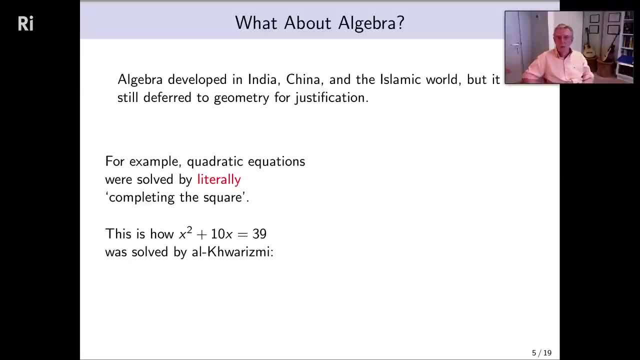 which is also very, very important For the rest of this story. as you will see Now, Al-Khwarizmi's algorithm for solving quadratic equations was like this: If we got the equation with x squared plus 10x on one side, 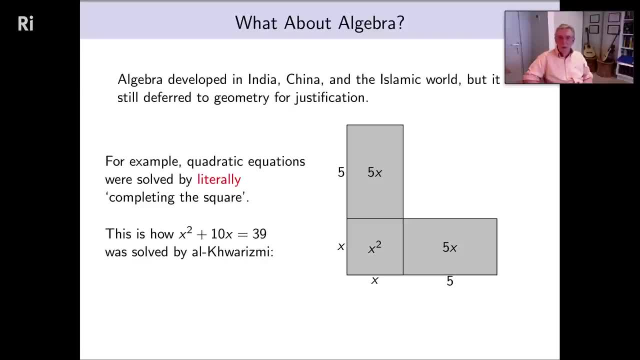 he views this as a square plus two rectangles. We would say the square is x squared the square with side equal to x. And he split the 10x into two pieces, a five x and a five x. One of them has width five and height x. 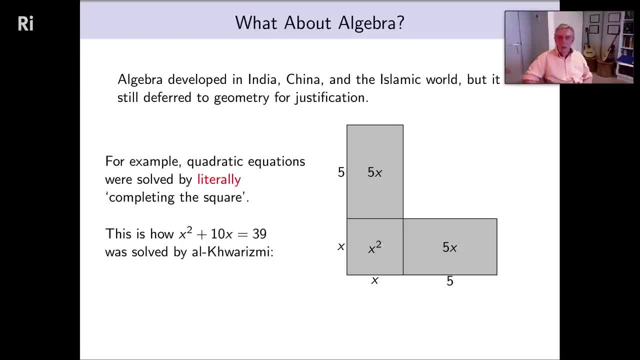 the other has height five and width x. So these three objects together make an L-shaped piece, which the right hand side tells us is equal to 39. Now, when you look at that L shape, it's just dying to be completed to a square. 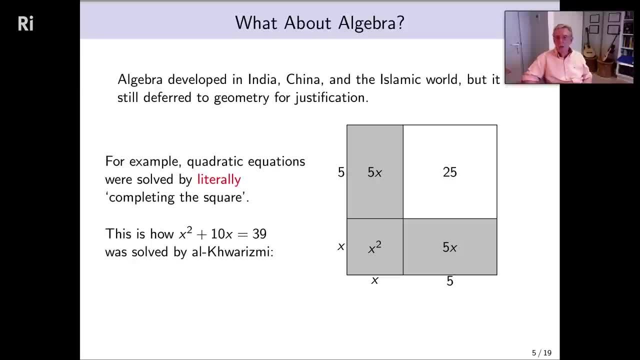 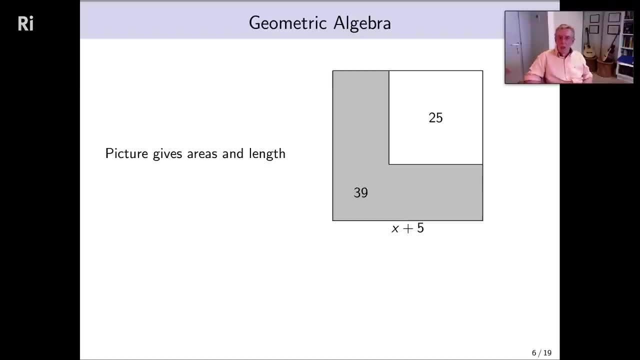 And the square has width five and height five, So it has area 25.. There it is, And when we've completed the square, we have basically this picture: An L-shaped area of size 39, a square of size 25.. 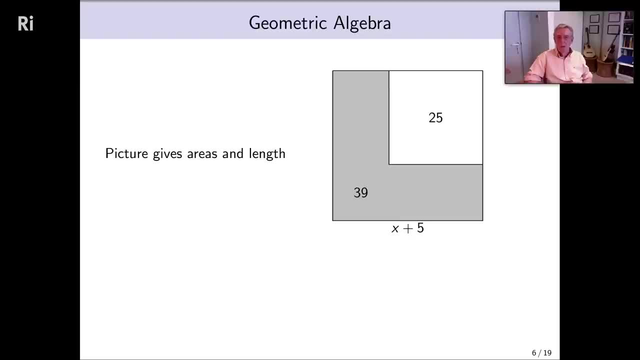 The width is x plus five. That was the square plus the width of the rectangle. But 39 plus 25 is 64, which is the square of eight. So this completed square is a square of width eight, which is also equal to x plus five. 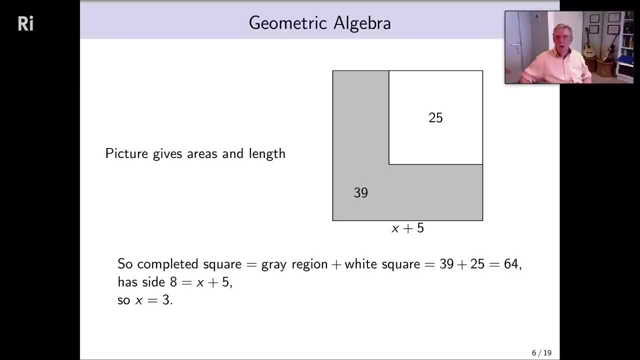 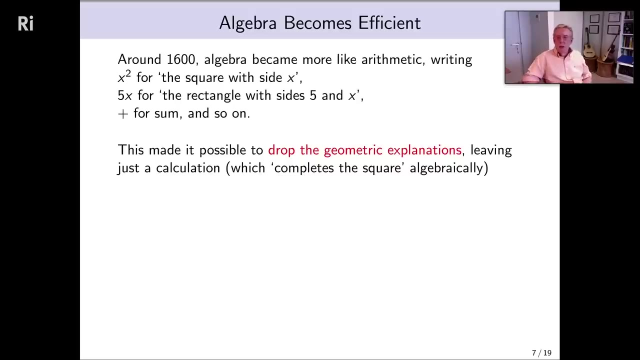 Therefore x equals three. We've solved the quadratic equation by pure geometry. He didn't have the symbol x or x squared or five x. He just drew this picture. Now, it wasn't until around 1600 that people started to do algebra the way we do it today. 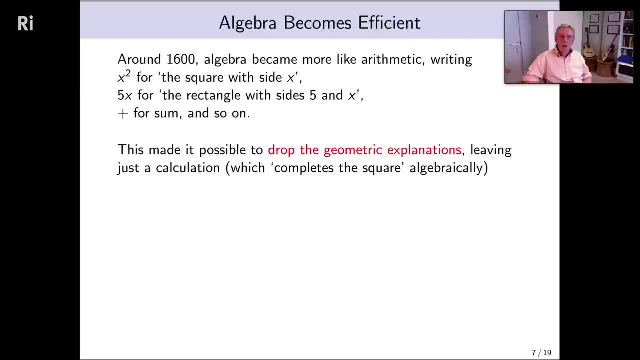 which is more like arithmetic. People realized you could write x squared but the superscript two to denote the square with side x and five, x for the rectangle with sides five and x and a plus sign for the sum and so forth, And it became very efficient to deal with squares. 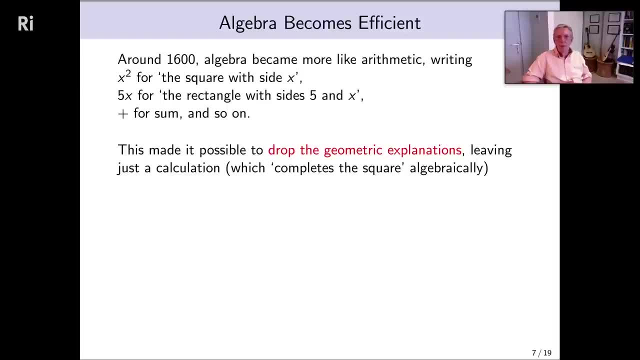 and rectangles simply by arithmetic operations: plus and minus and multiplication. So it became possible to completely drop the geometric explanations, leaving just the calculation, Like this one, And this is what Al-Khrizmyi did with squares and rectangles, done with symbols: the x squared the 10x. 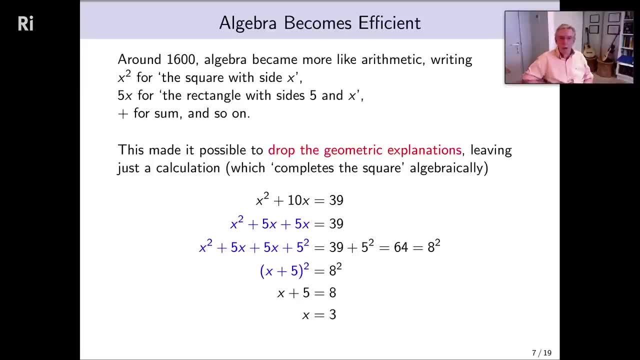 And the completing, the square bit I've highlighted in blue. And if you're inclined to think geometrically, you probably think this is not as clear as looking at squares and rectangles, and maybe it isn't, But nevertheless, people got used to it. 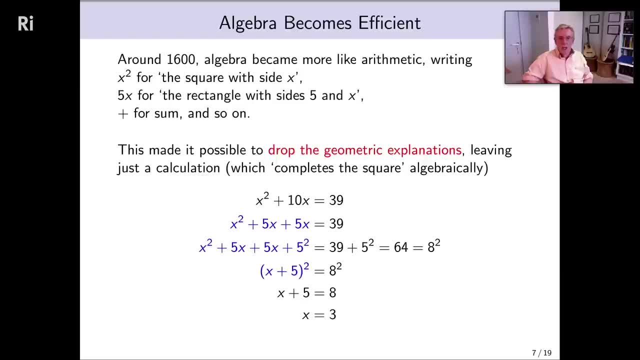 And they got used to seeing that x squared plus five, x plus five, x plus five squared is the square of x plus five. so completing the square could be done by algebraic recognition rather than geometric recognition, and it was more efficient if you could just write things down like this: 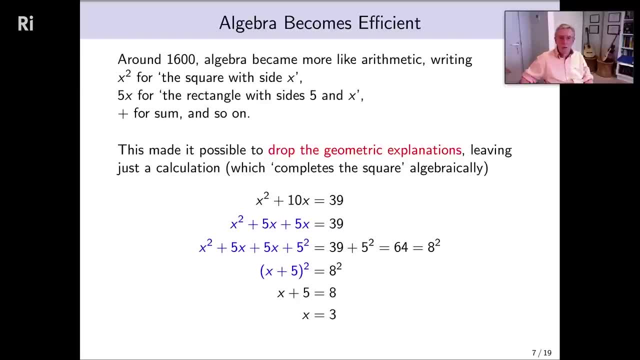 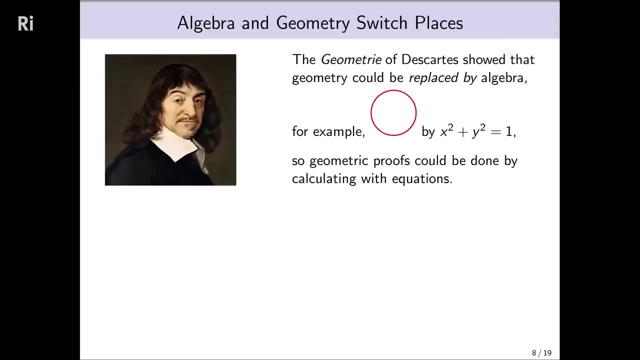 without having to draw pictures of squares and rectangles, and this led to a kind of takeover of geometry by algebra and Descartes. was is, of course, famous for doing this. in his geometry 1637, for instance, instead of drawing a circle, you could write down the equation: x squared plus y squared equals one, which denotes a circle with radius one. 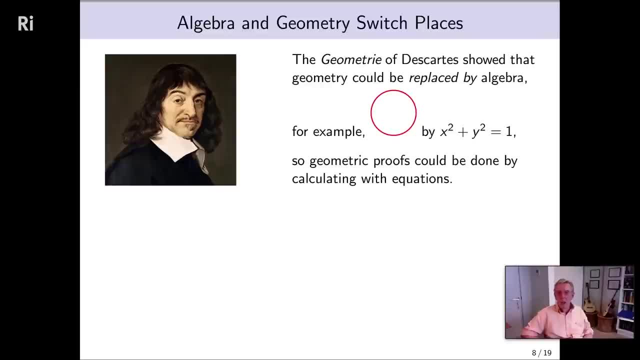 instead of drawing a straight line, you could write down a linear equation, which is why they we call them linear, incidentally. and if you wanted to find where the line intersects the circle, you could simultaneously solve the equation of the circle and the equation of the line. so, all in all, anything that Euclid did could be done by calculating with equations. 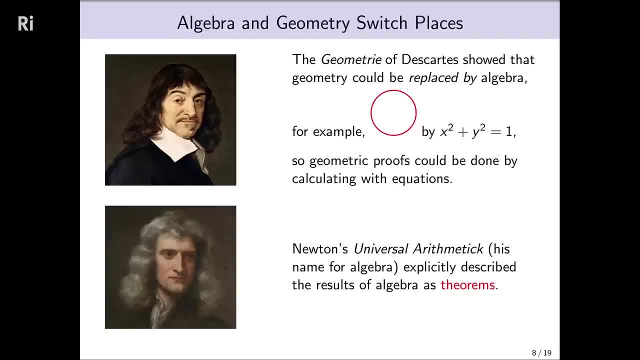 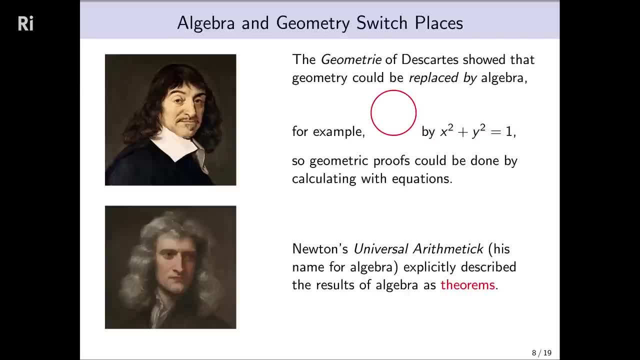 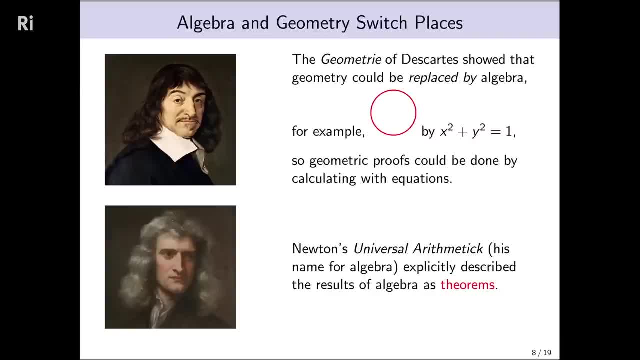 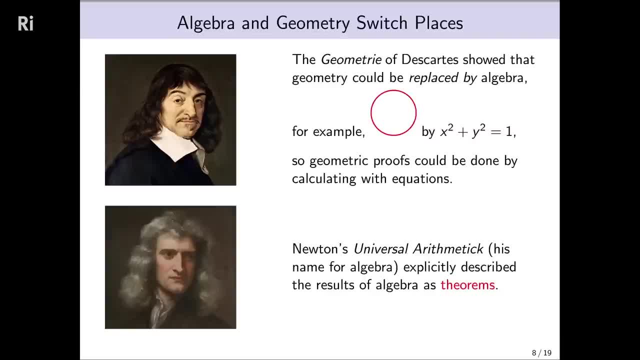 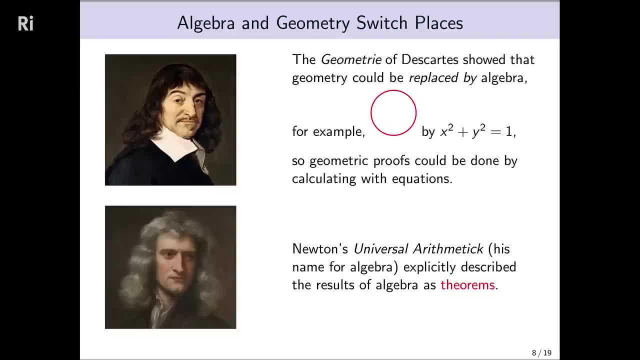 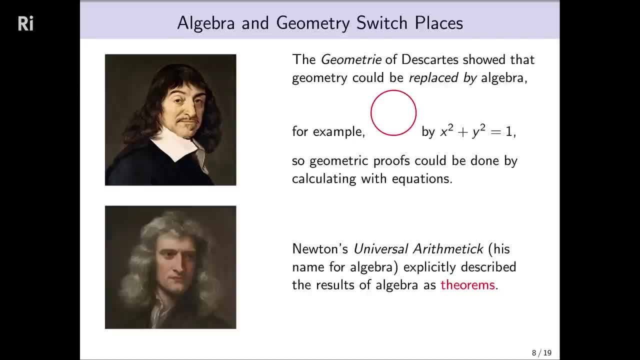 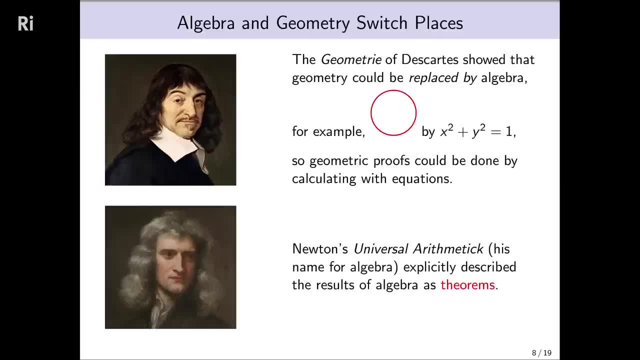 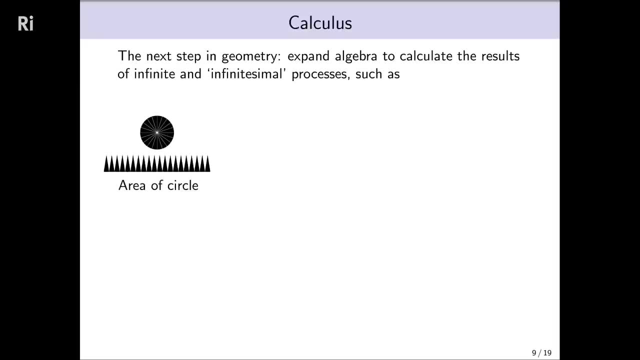 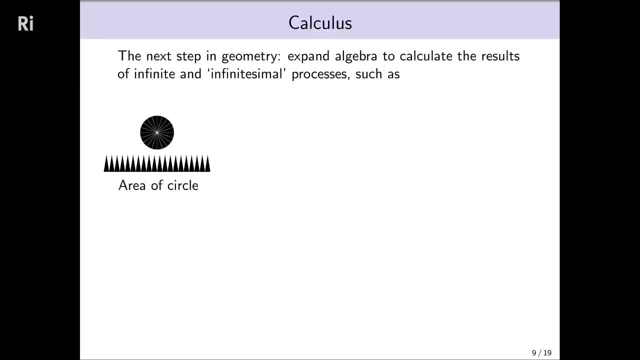 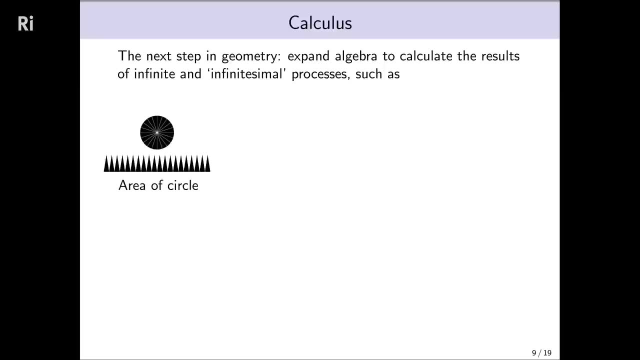 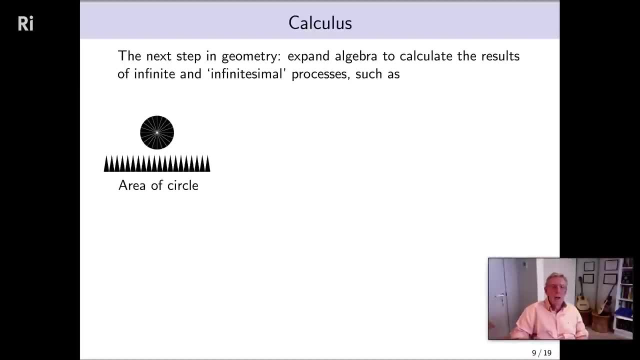 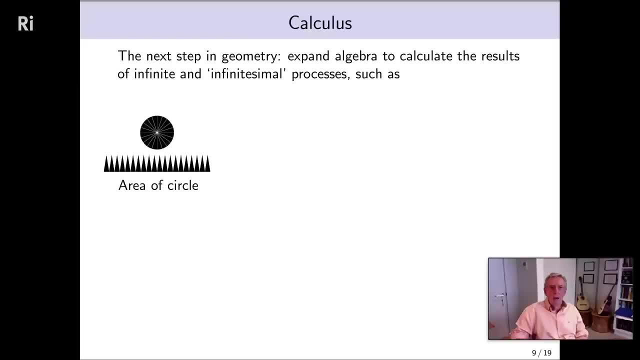 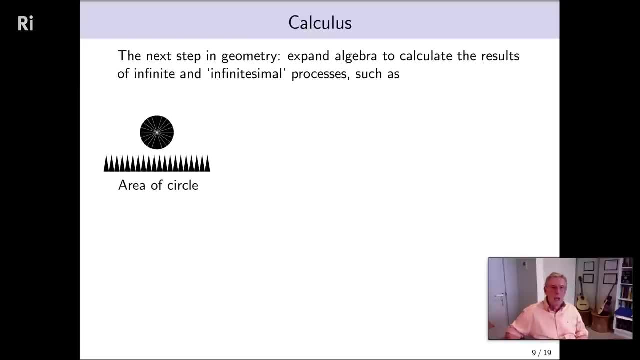 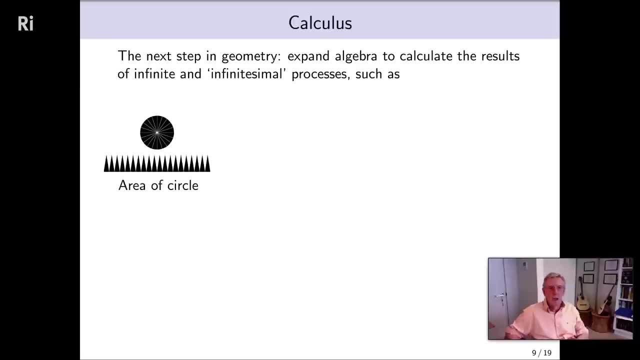 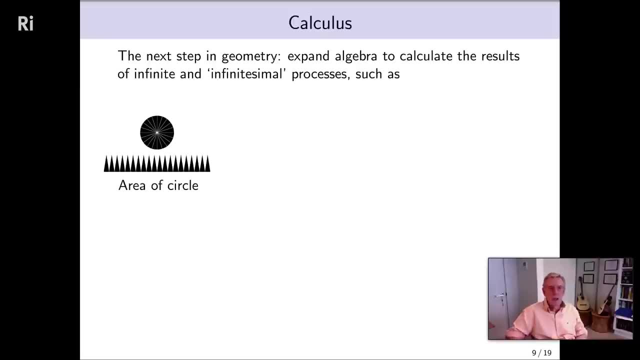 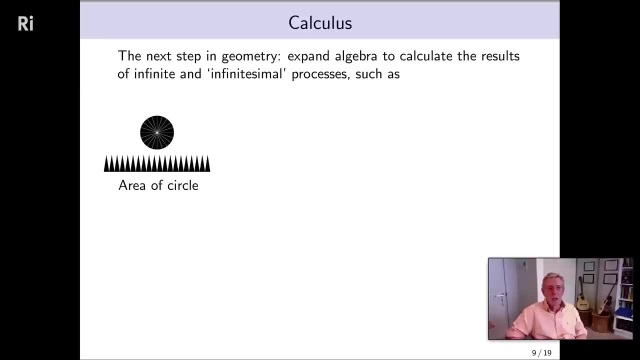 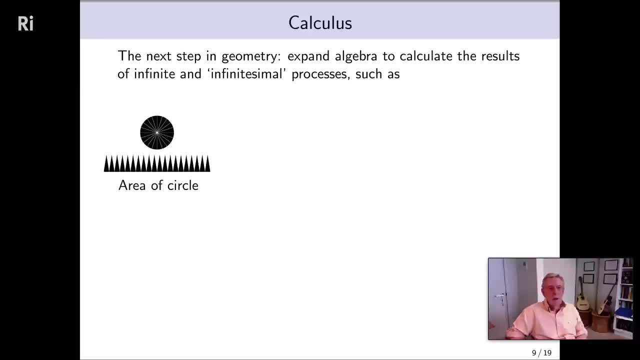 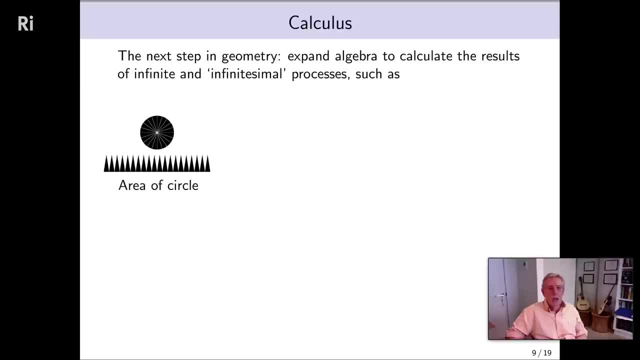 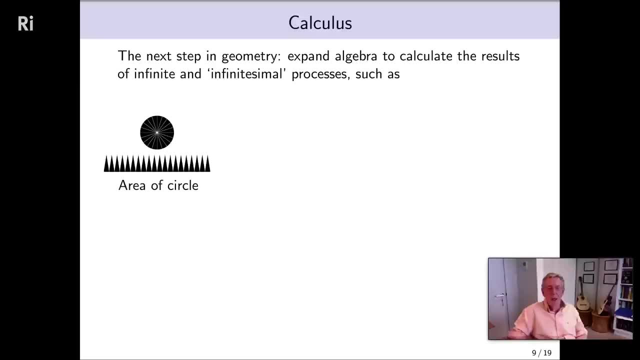 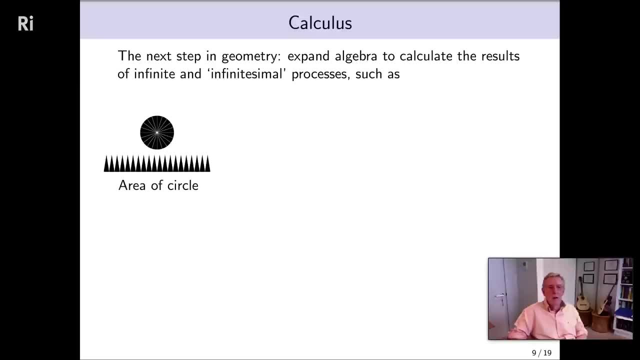 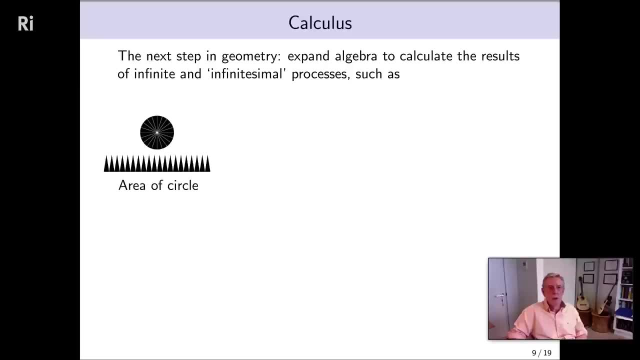 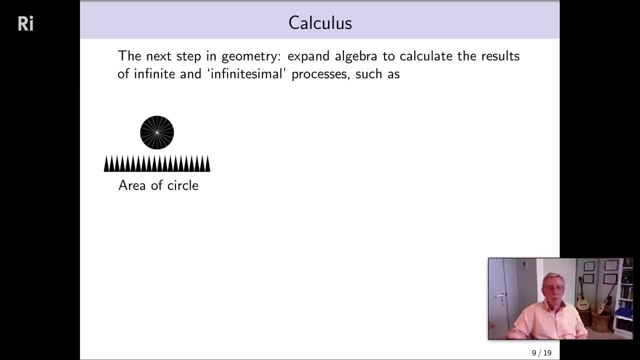 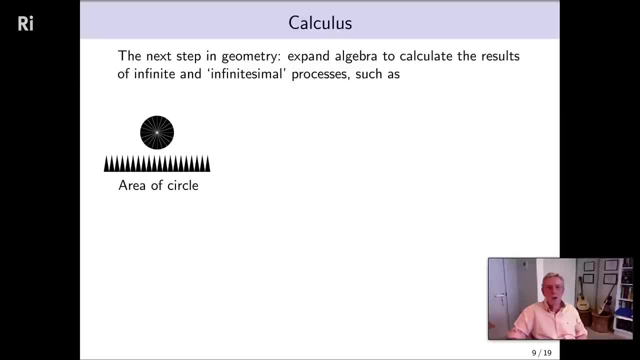 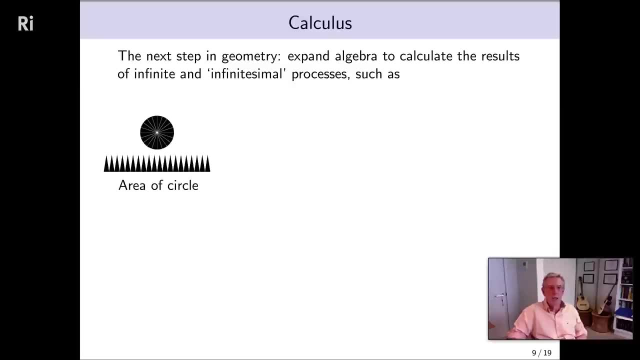 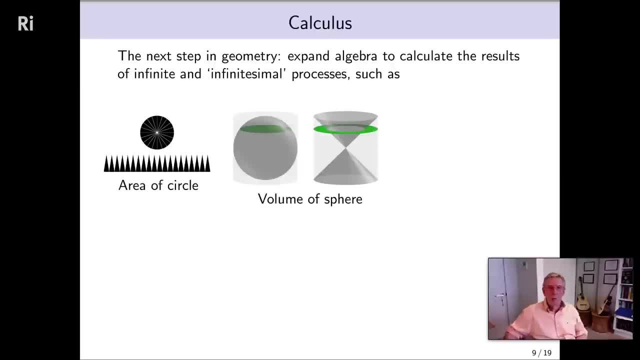 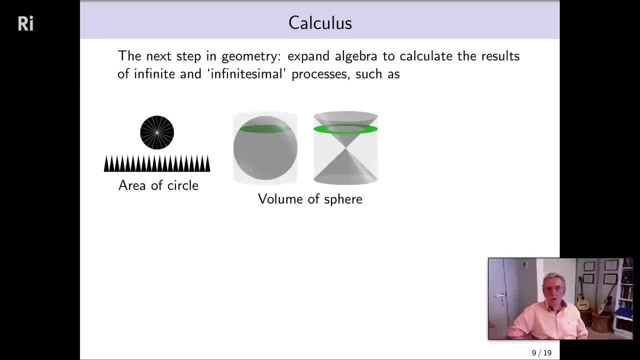 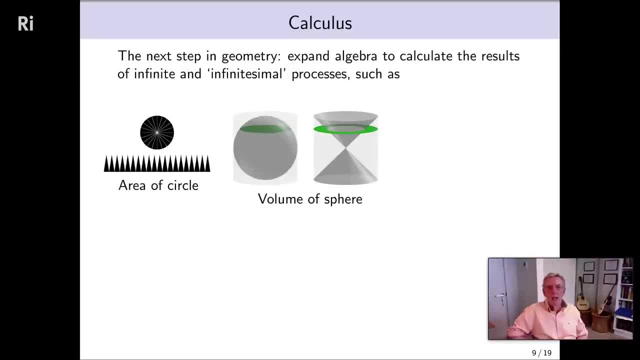 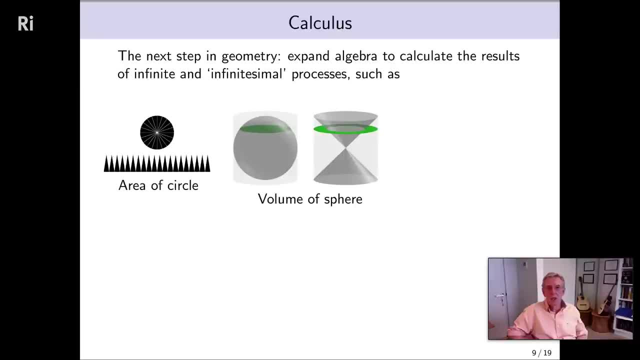 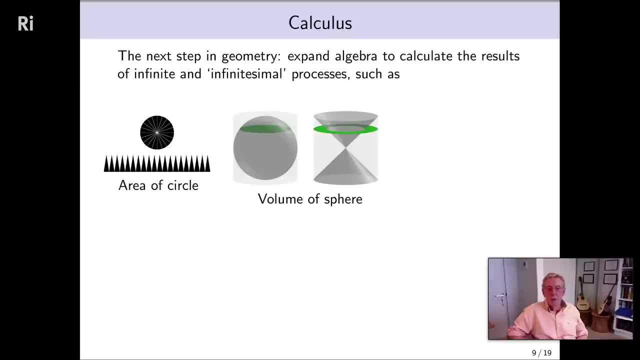 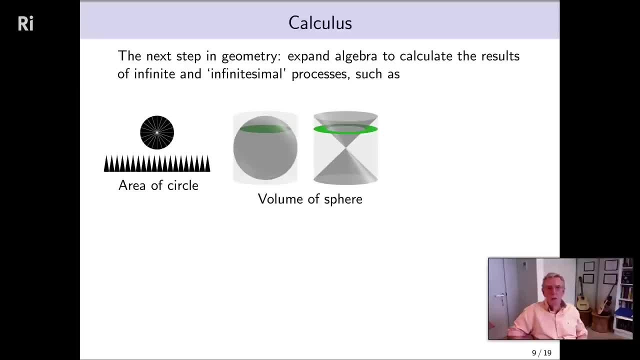 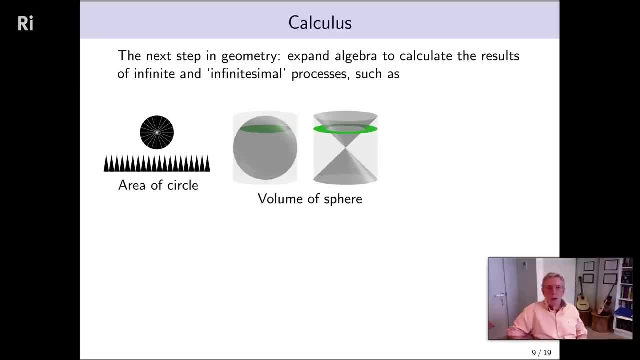 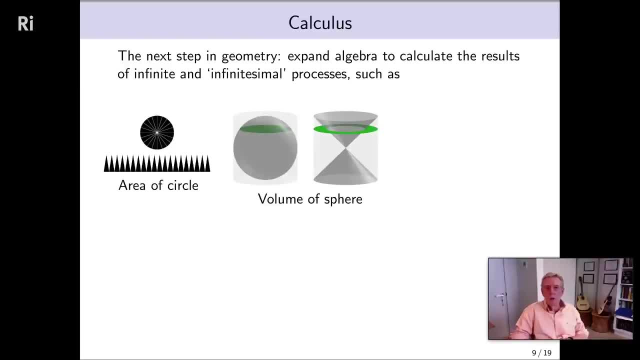 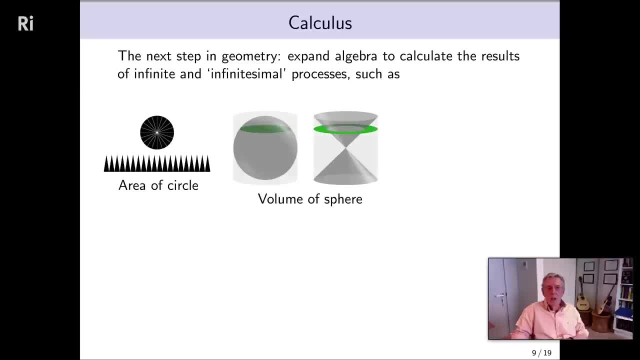 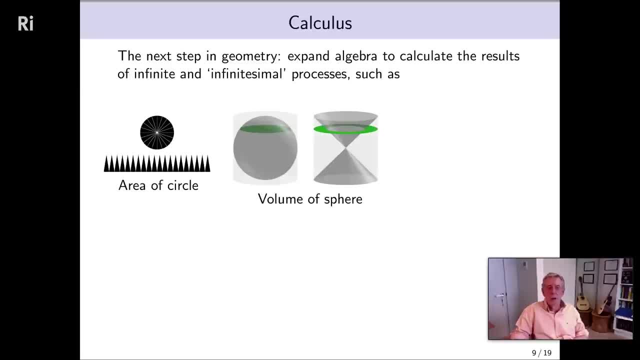 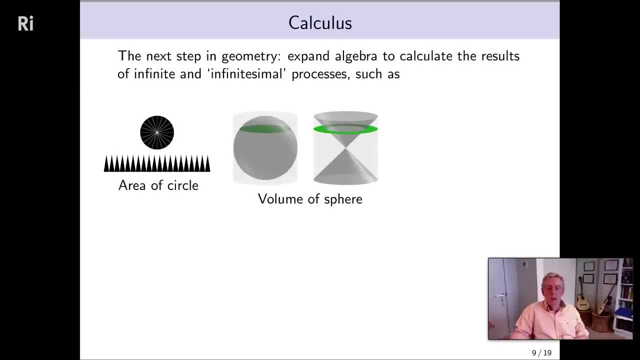 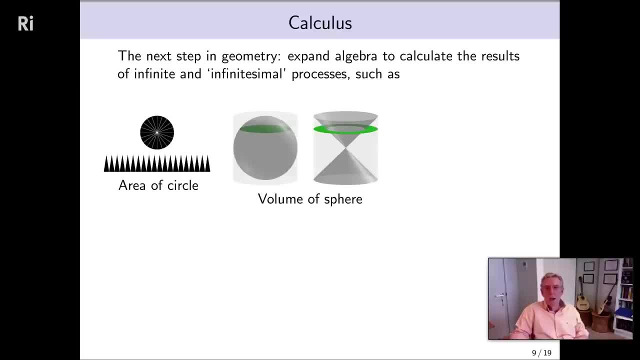 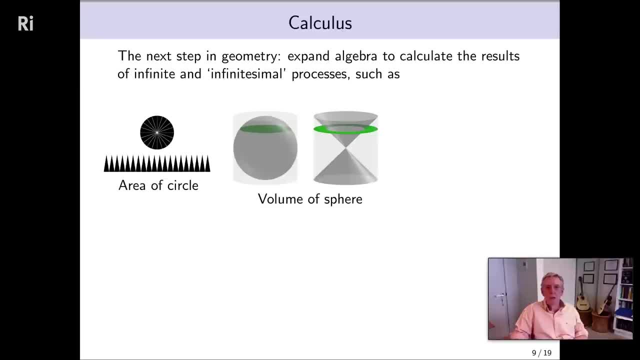 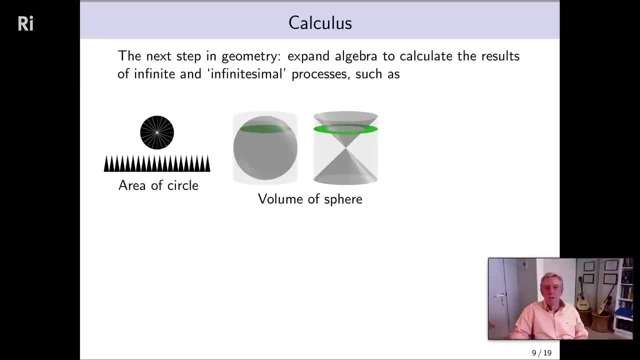 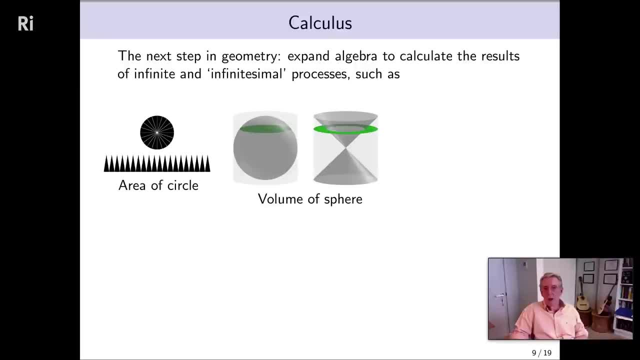 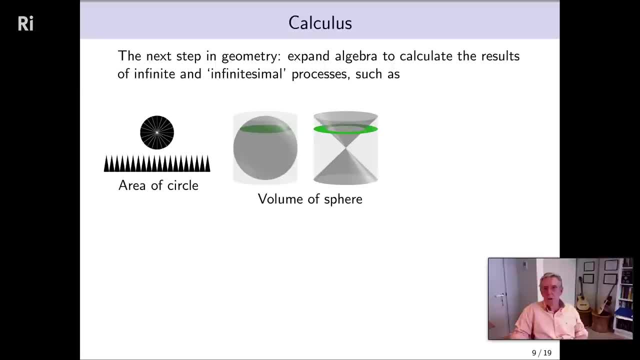 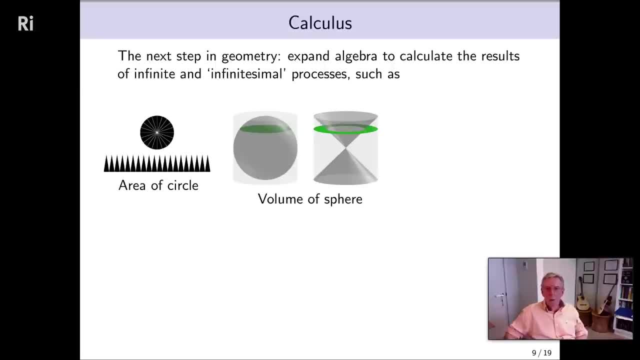 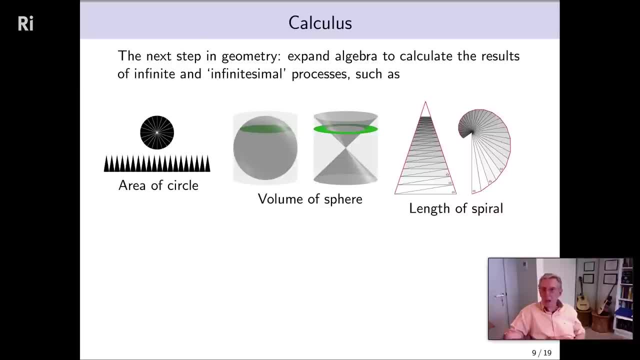 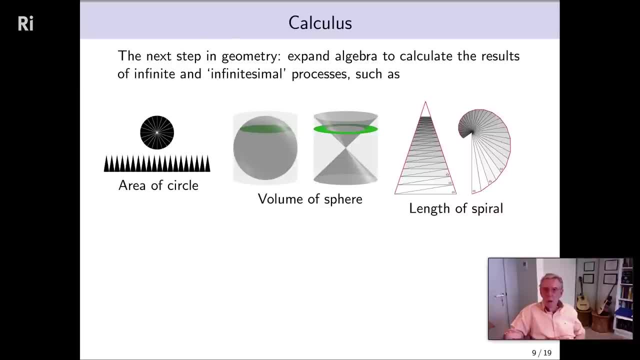 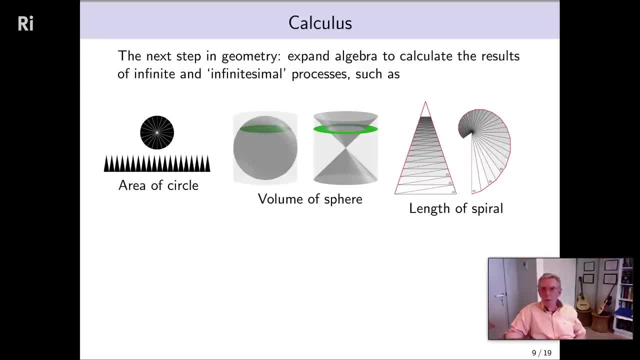 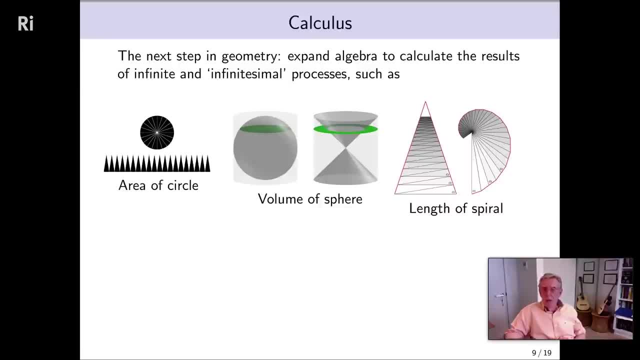 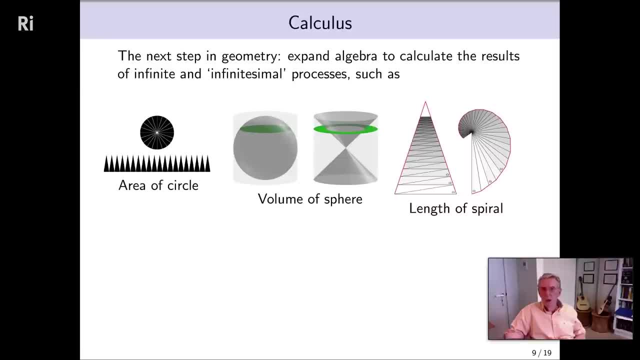 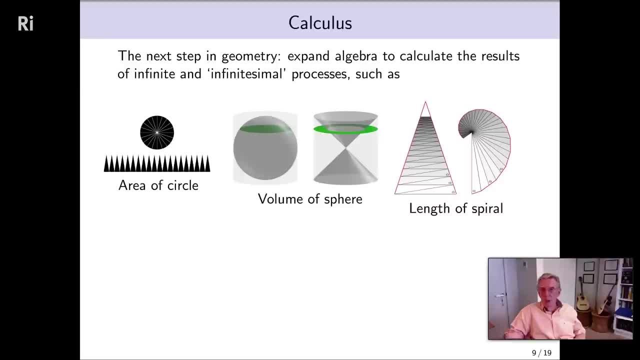 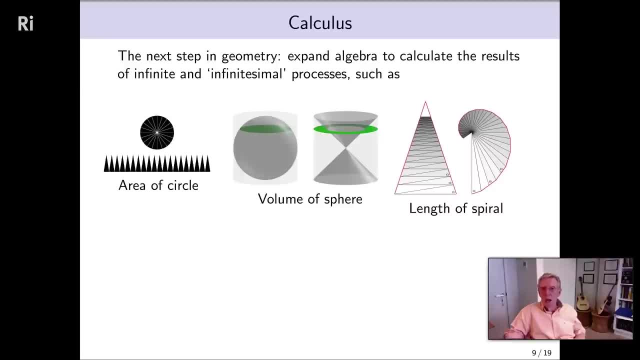 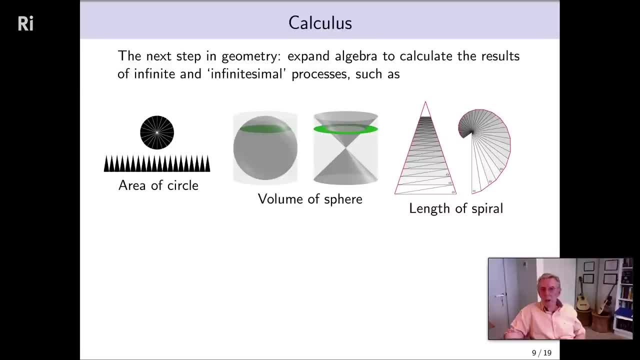 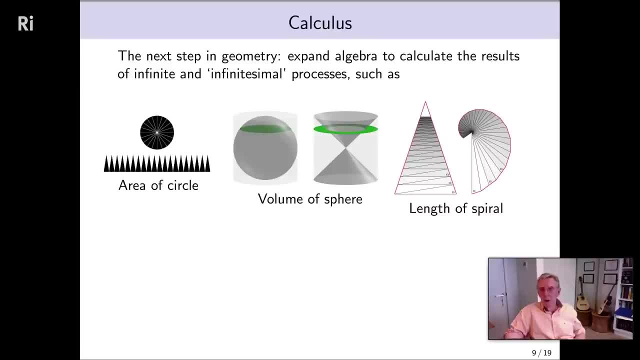 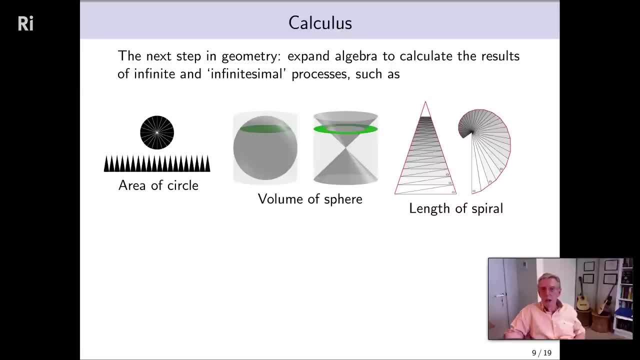 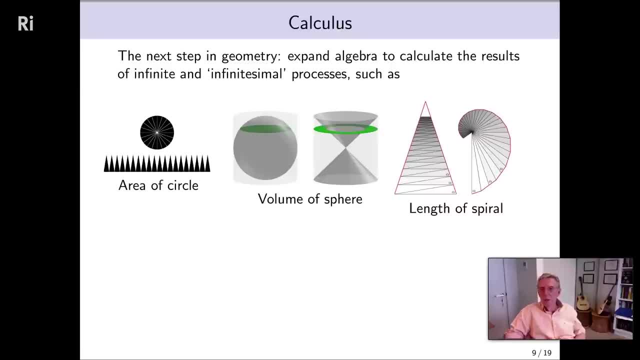 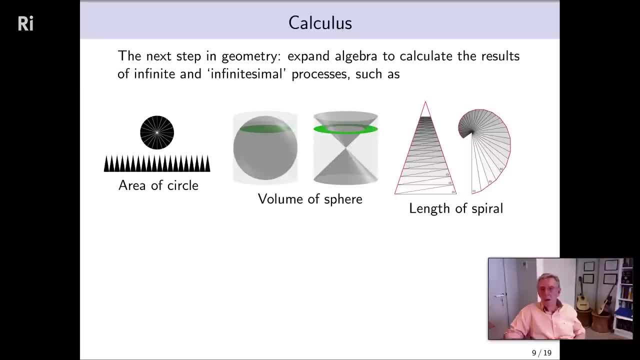 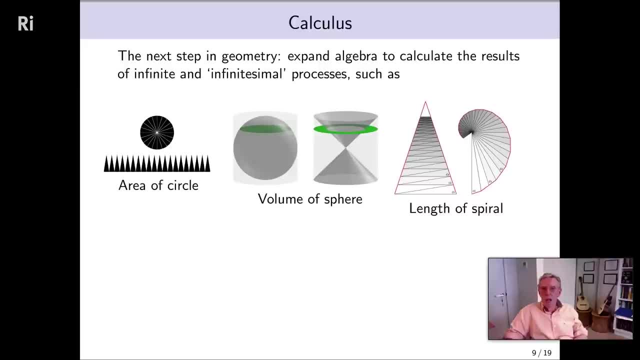 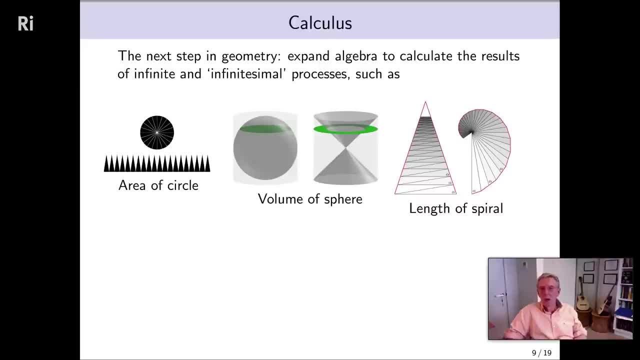 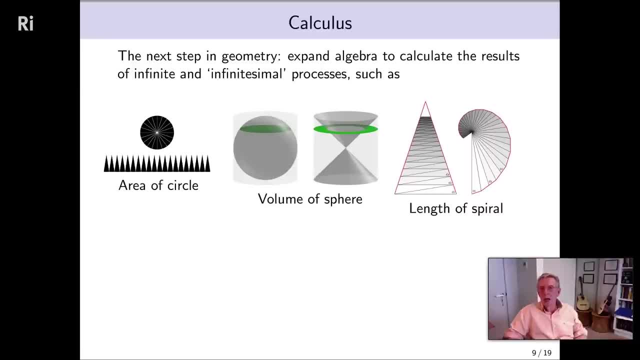 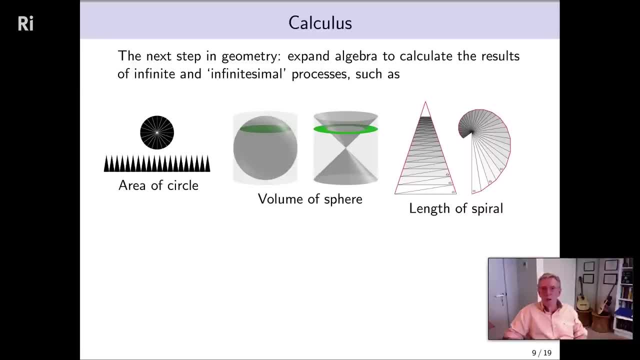 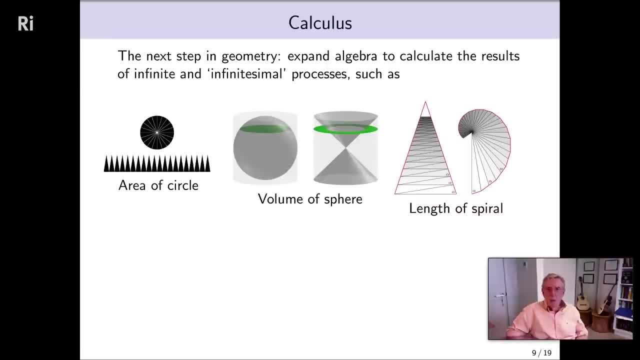 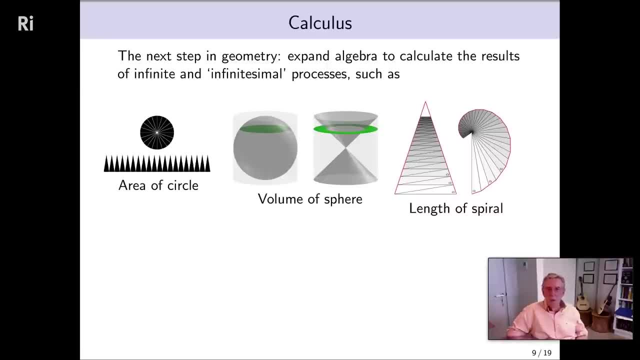 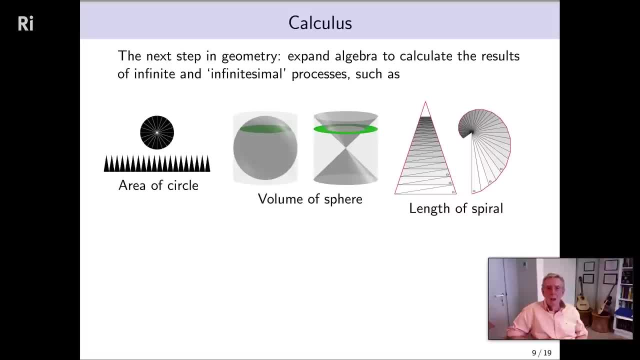 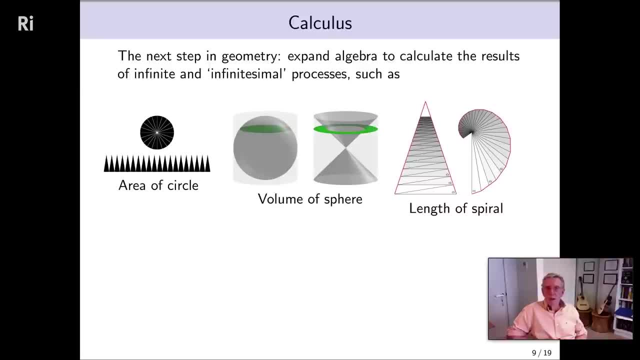 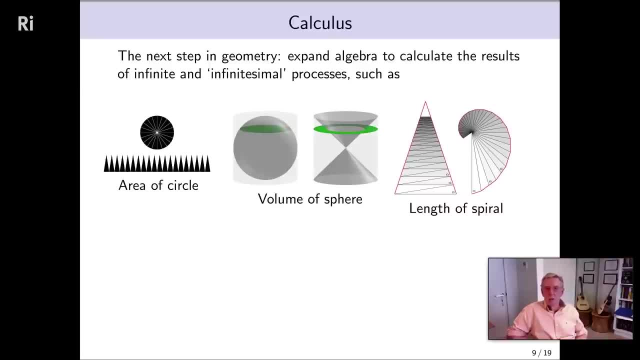 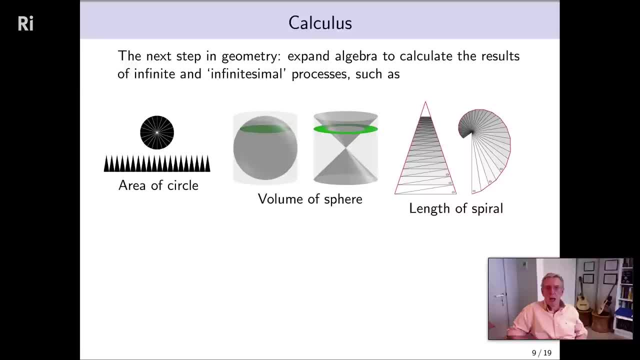 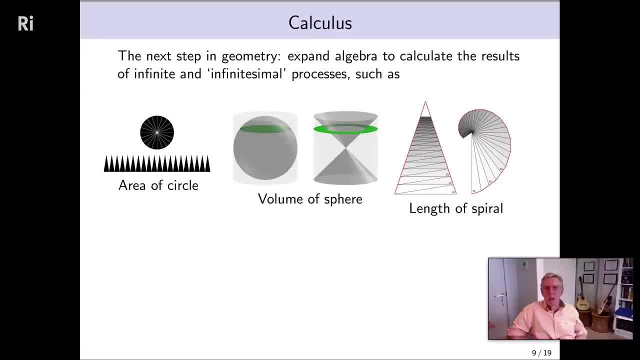 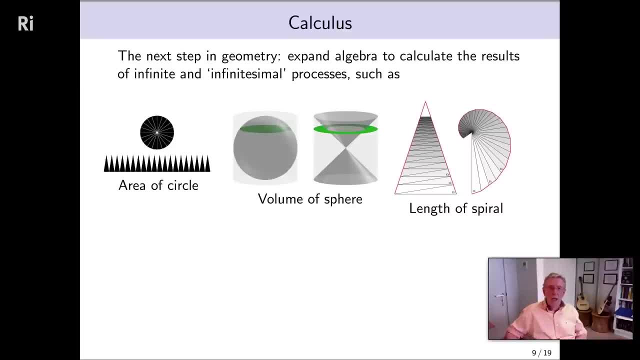 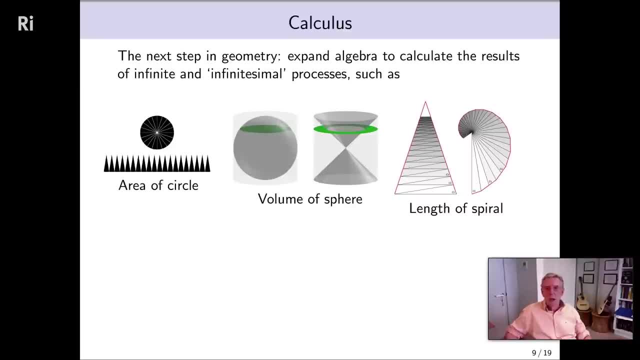 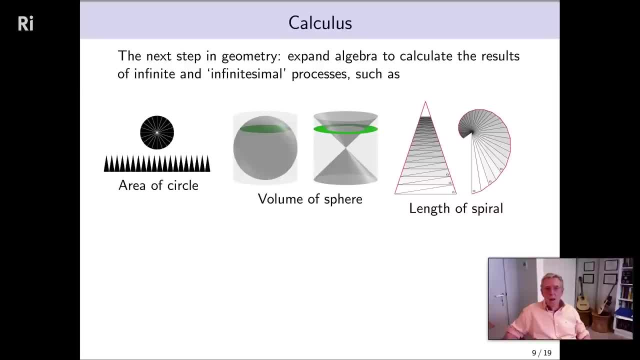 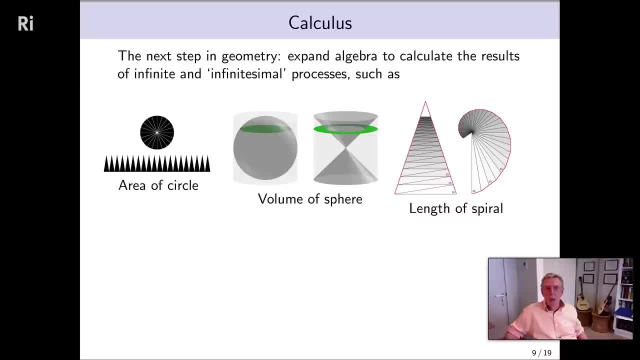 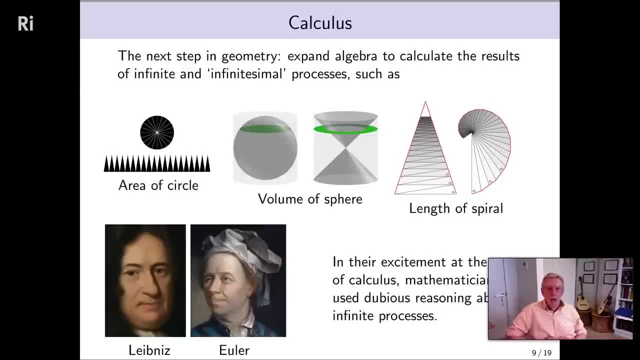 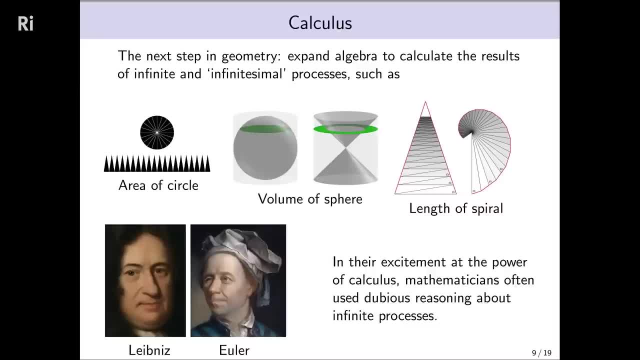 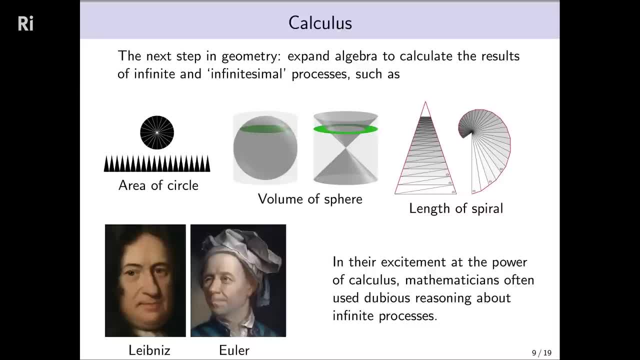 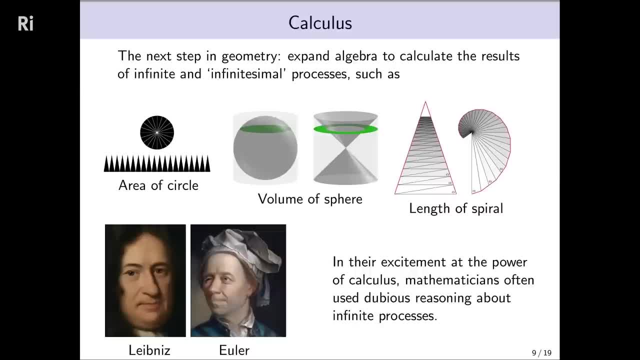 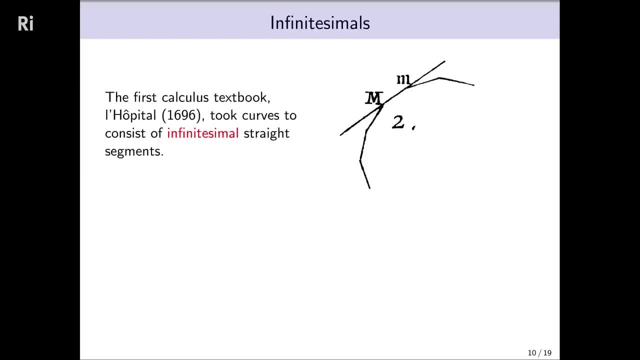 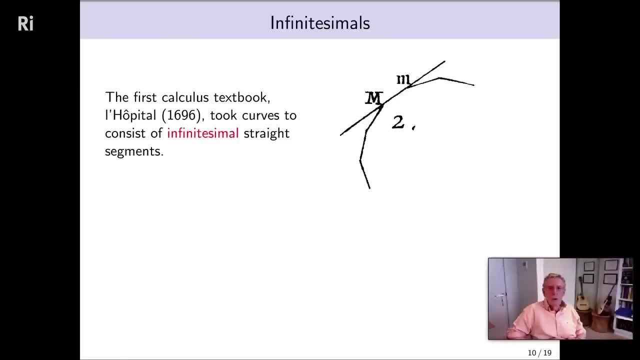 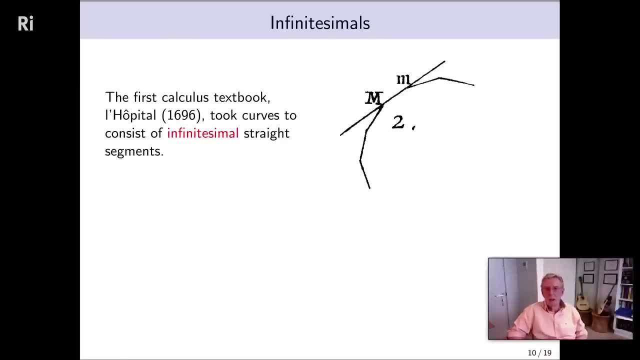 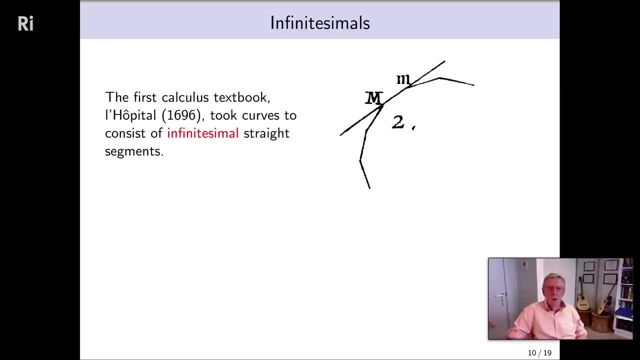 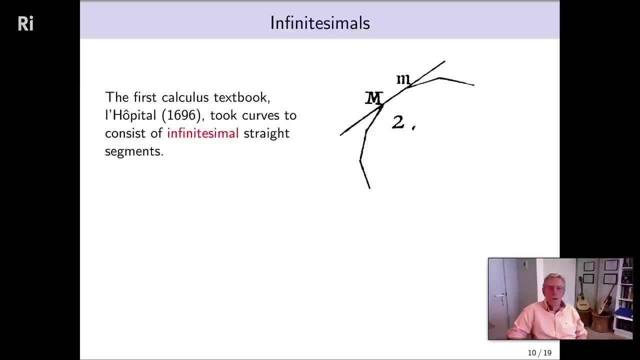 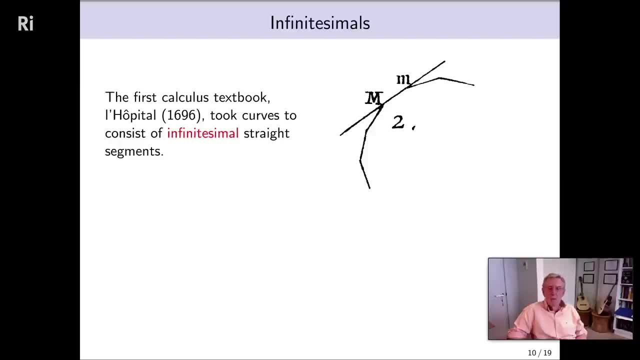 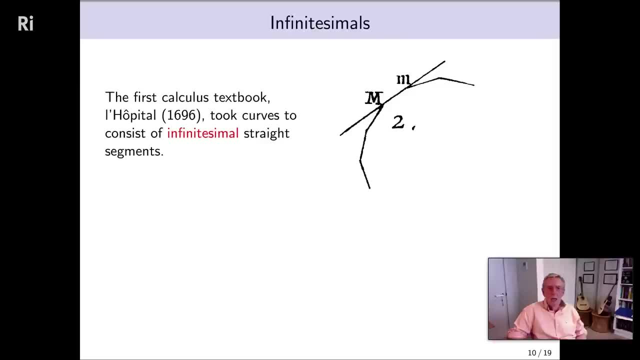 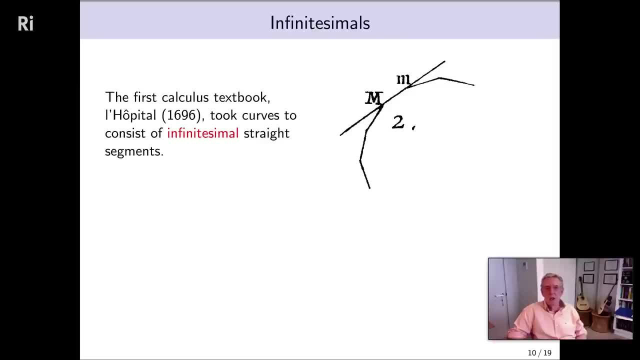 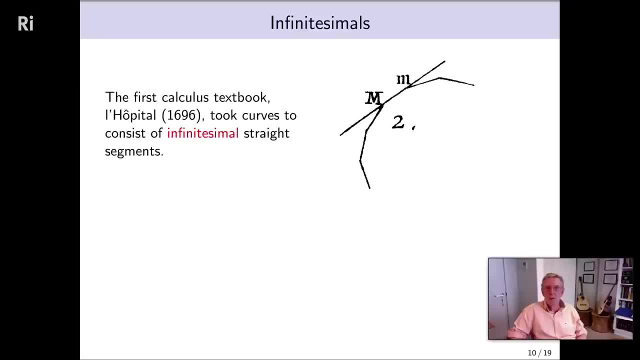 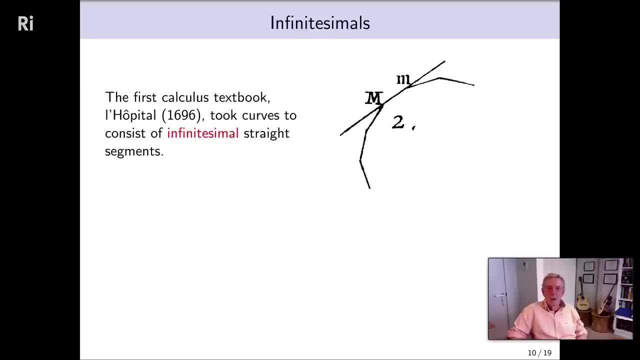 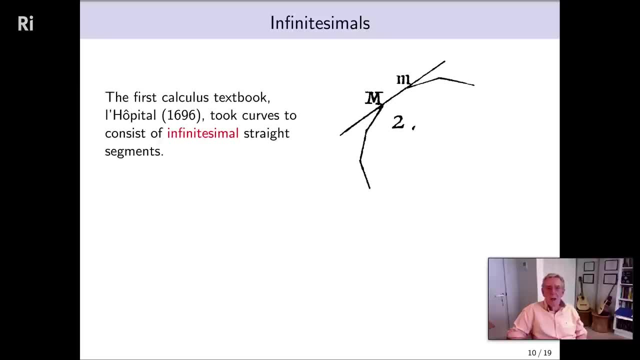 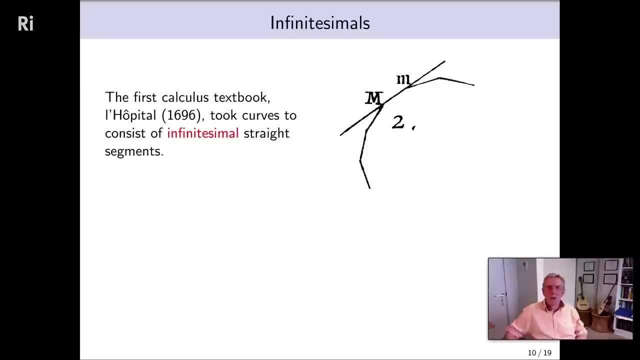 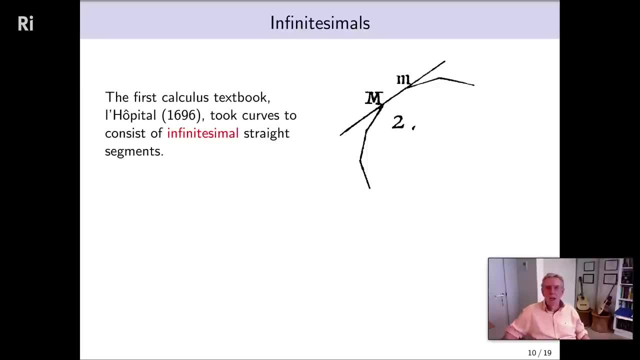 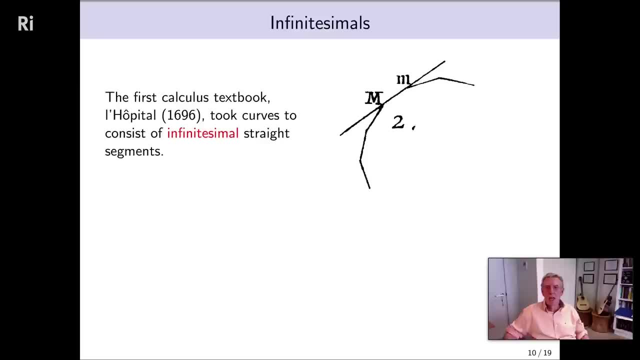 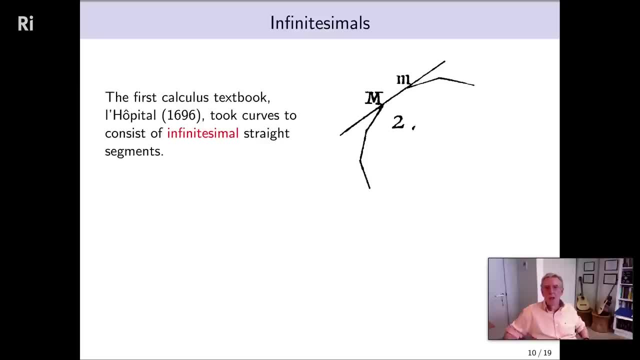 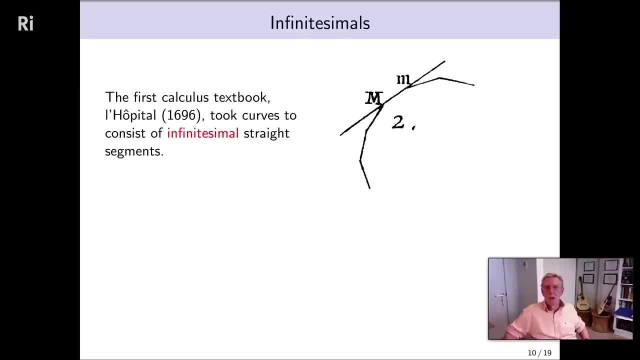 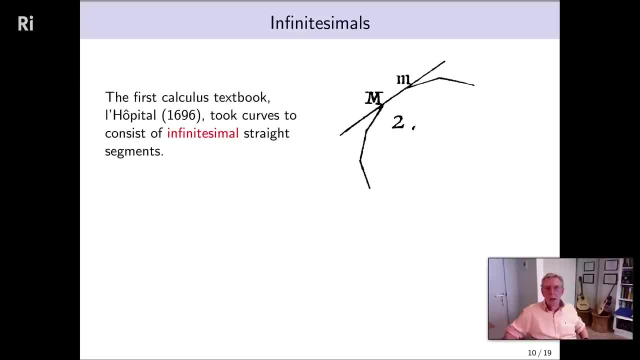 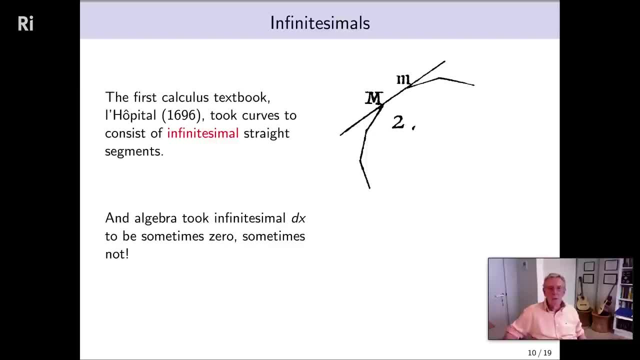 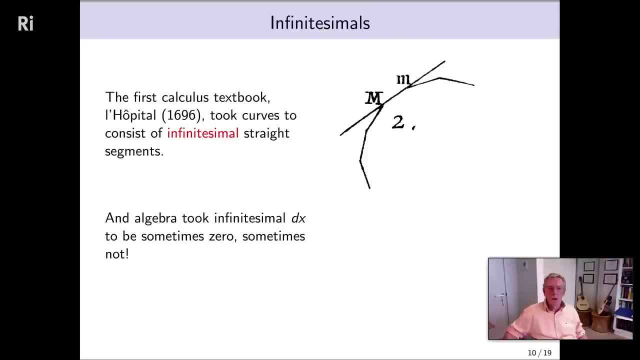 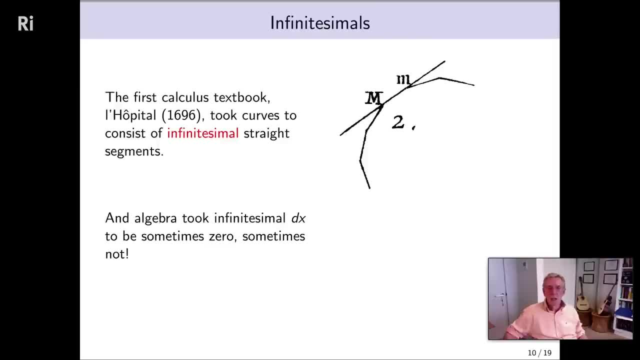 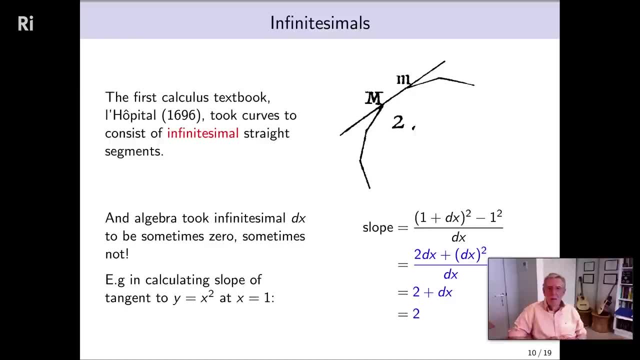 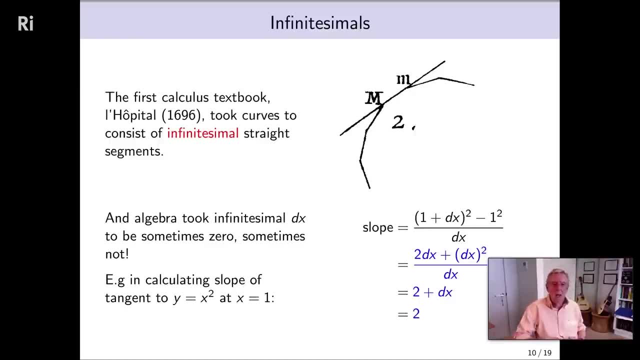 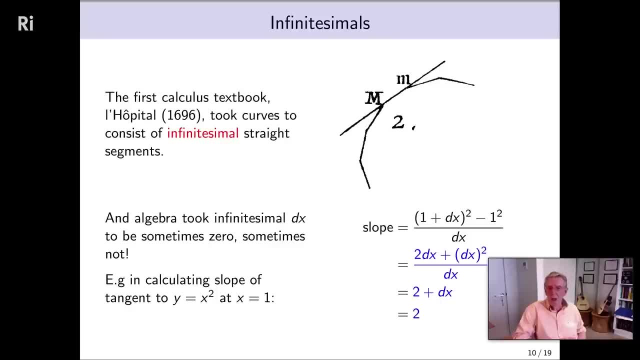 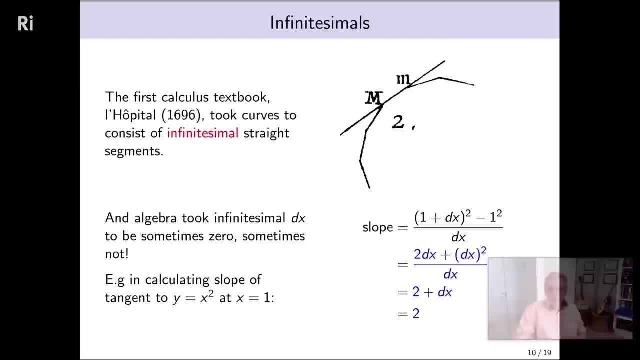 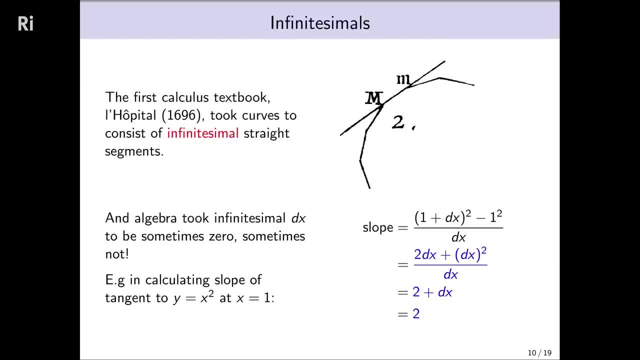 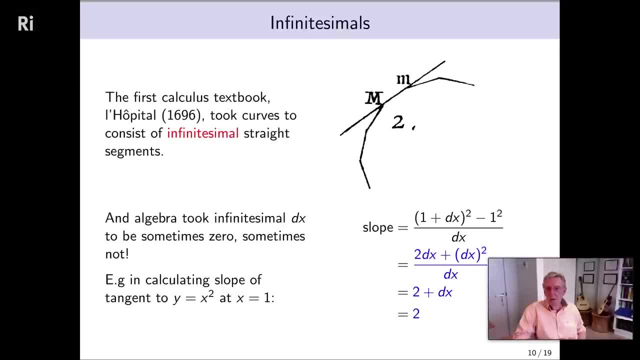 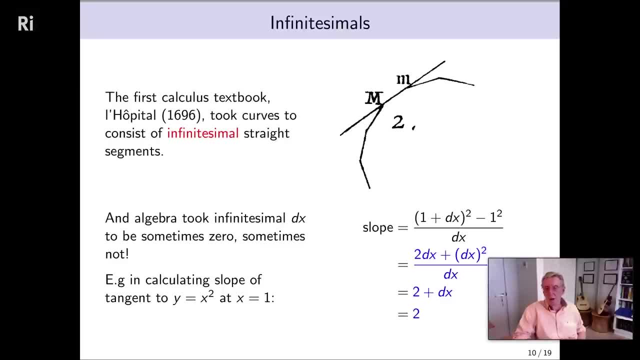 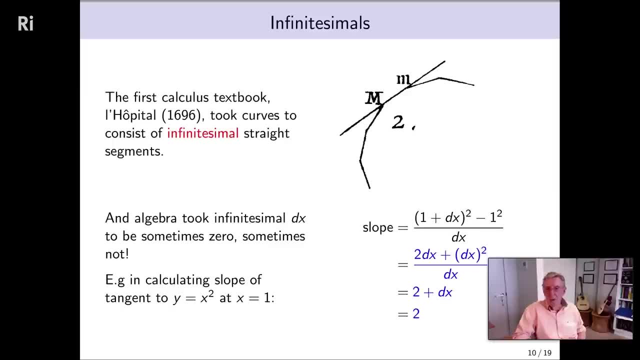 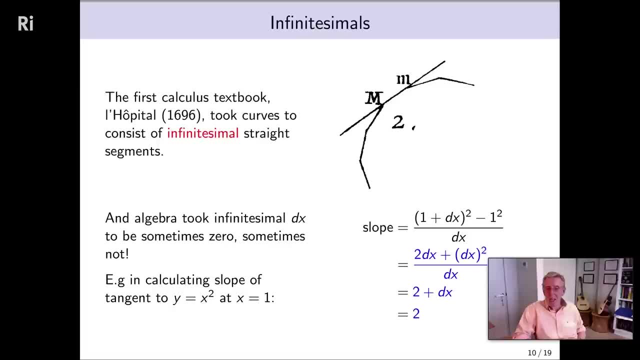 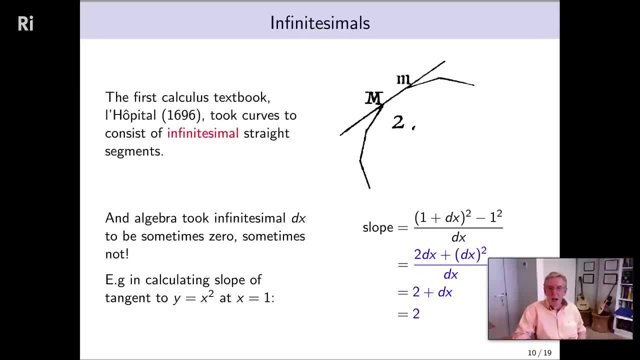 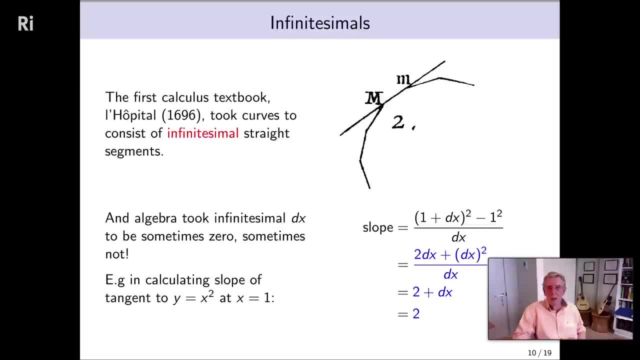 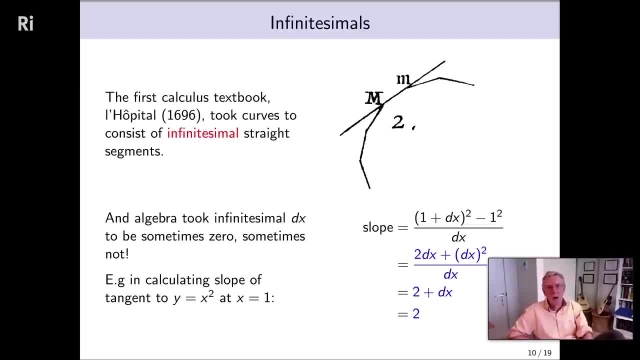 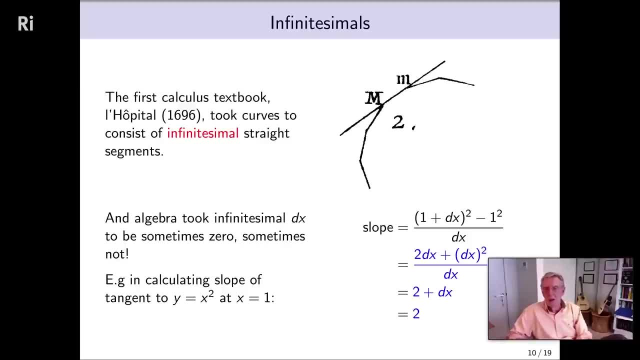 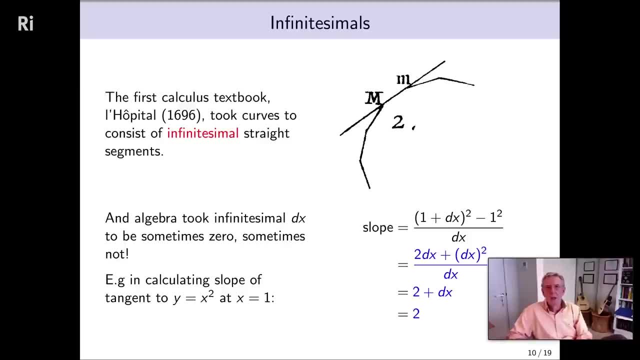 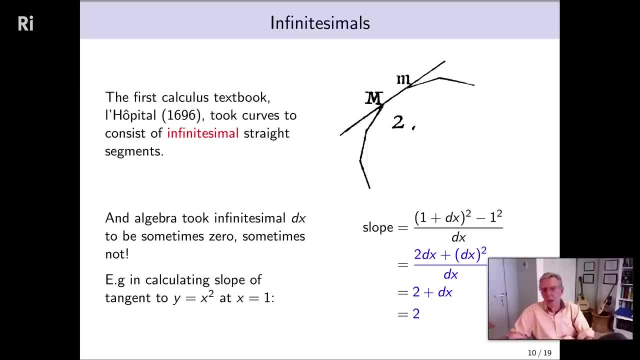 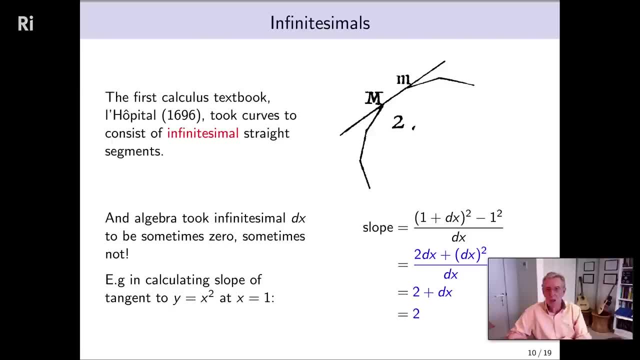 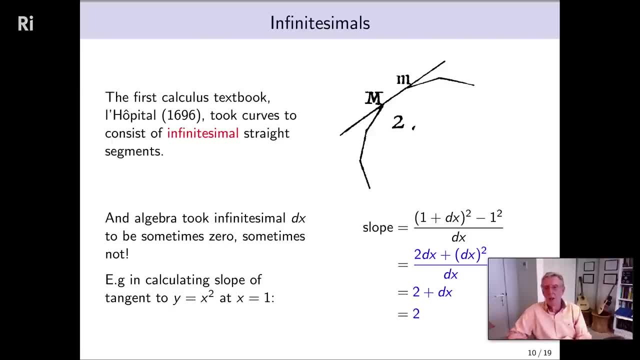 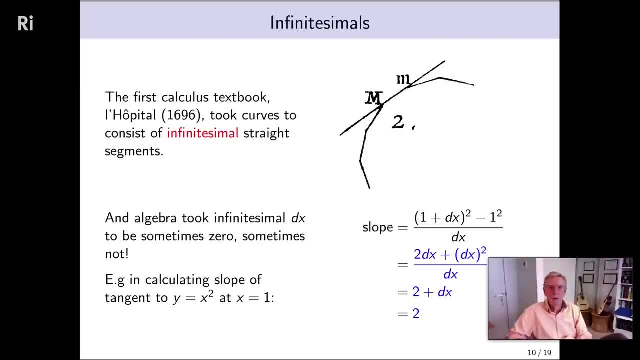 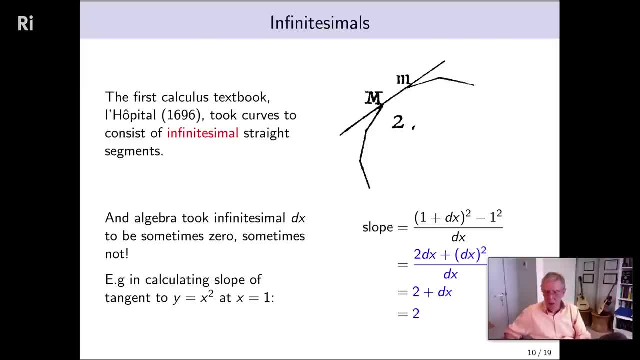 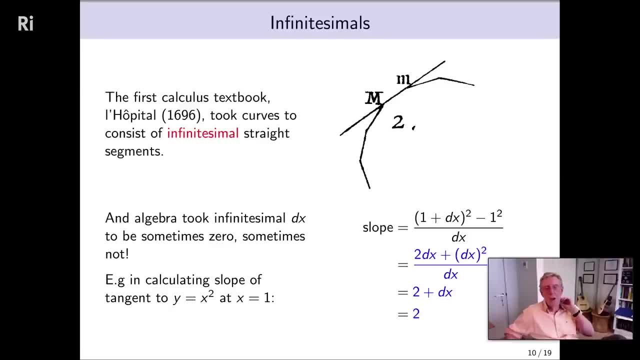 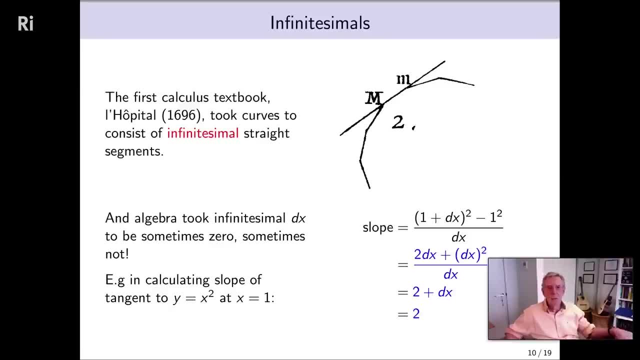 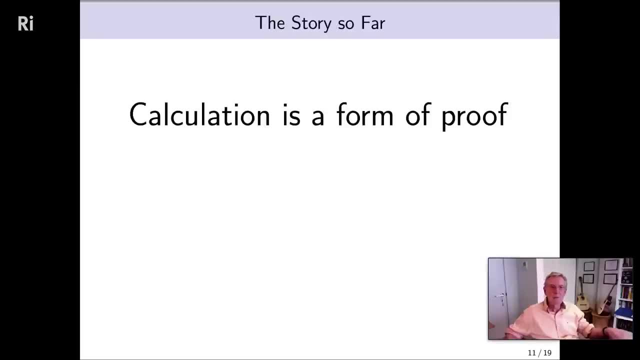 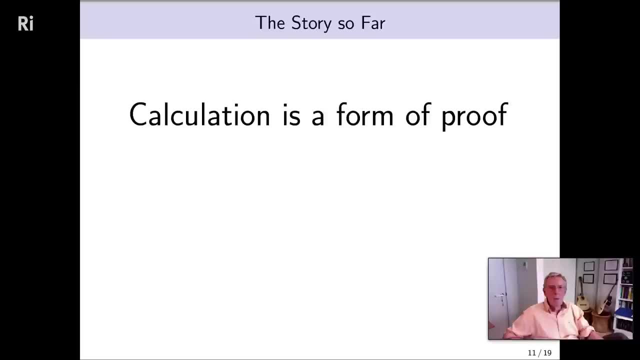 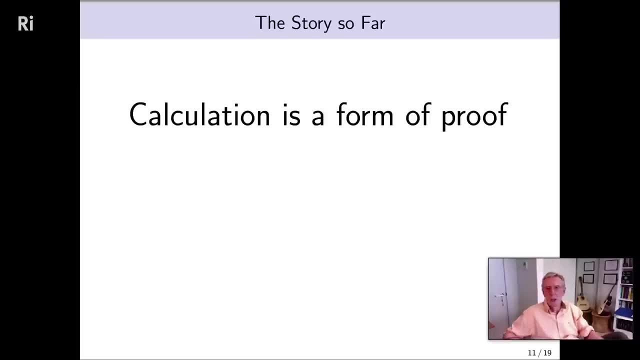 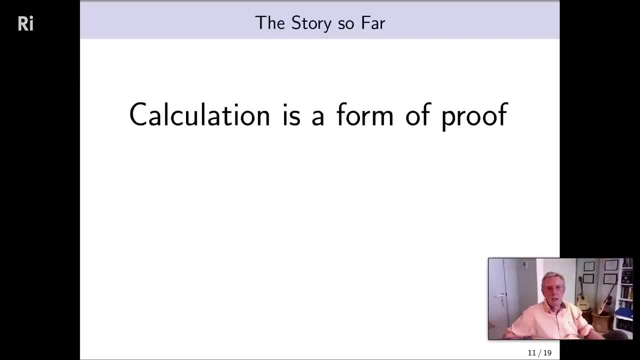 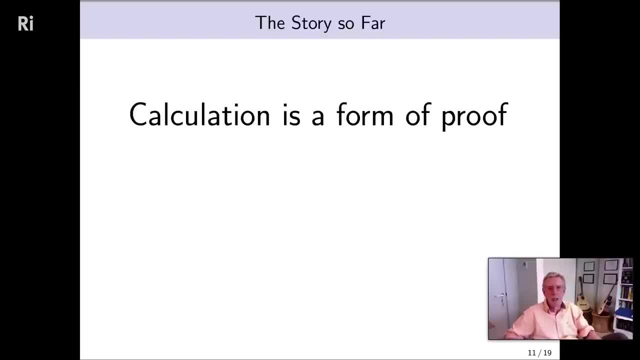 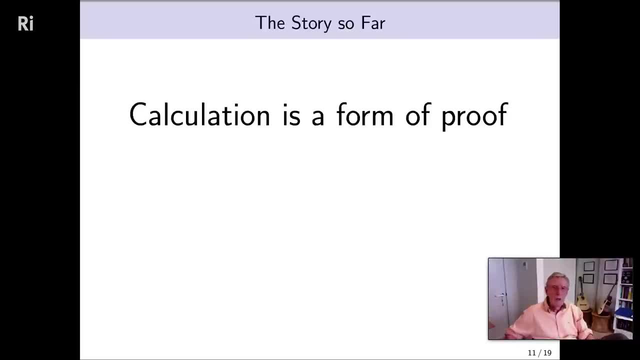 of proof and ingenuity. so calculation as i said it's, it's not to be ridiculed or belittled. it is a form of proof and it is very powerful. but next i want to show that proof is a form of calculation. this is the other side of the coin. now, the first to have the idea that logic could be done by 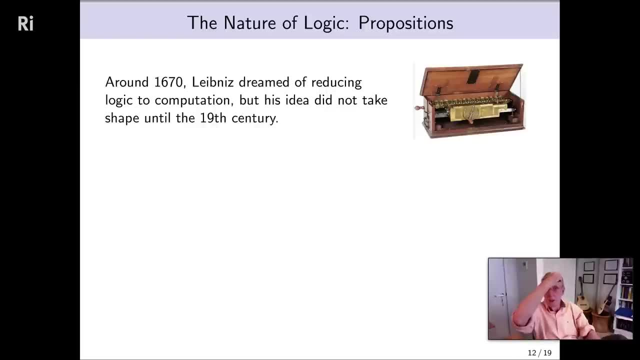 calculation was leibniz, and leibniz knew something about computation. he even designed a calculating machine- this is a picture of it which comes from a museum in hanover, which was where leibniz lived- and it was a machine that could add and multiply. so he knew something about it and he had this idea, that logic. 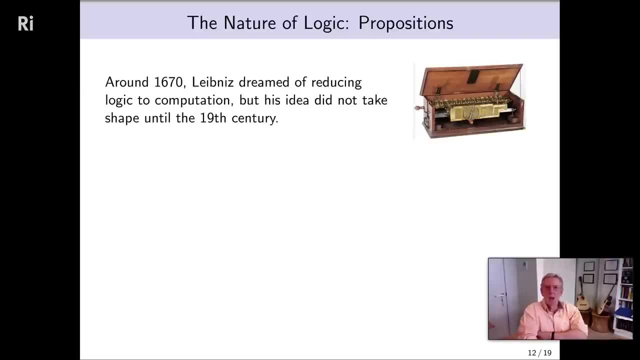 might be done by calculation and that sometime in the future it would be possible for people to settle arguments simply by saying, well, let us calculate and the calculation would show who was right. uh, but leibniz was a very busy man. he was a diplomat and a librarian and a philosopher. 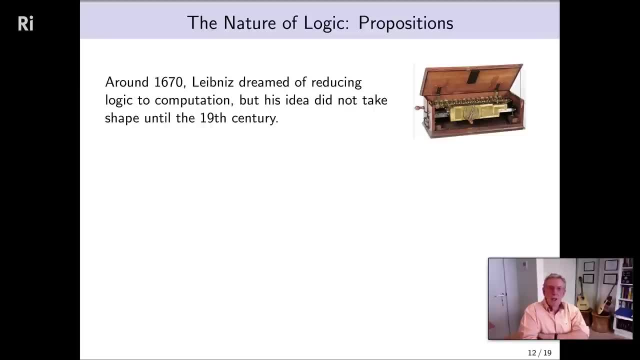 as well as being a mathematician, so he didn't get around to working out this idea in detail. uh, in fact, it didn't happen until the 19th century, a couple of centuries later, and the first important step in the process of reducing logic to computation was done by. 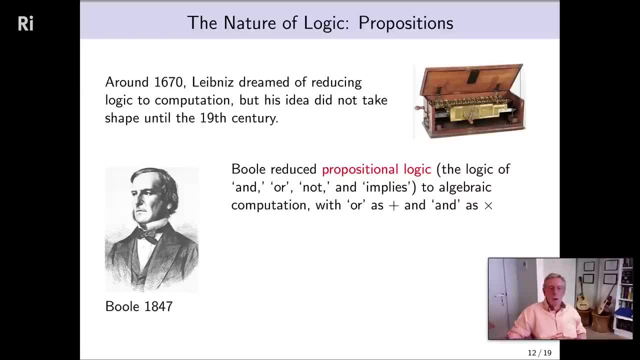 in 1847 and we now call what he did boolean algebra. it is a form of algebra and it it. it describes a certain part of logic called proposition logic. i mean propositional logic, um propositions are just denoted by letters, like in algebra, and the um the only attribute. 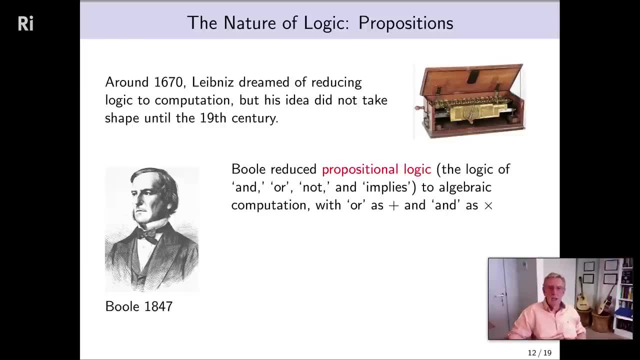 one of these letters has is either being true or false. it has a proposition. it's just those two values, true or false, and you combine propositions by words such as and or not, implies and boolean. you notice that uh, or was rather like the plus operation and was like modification. 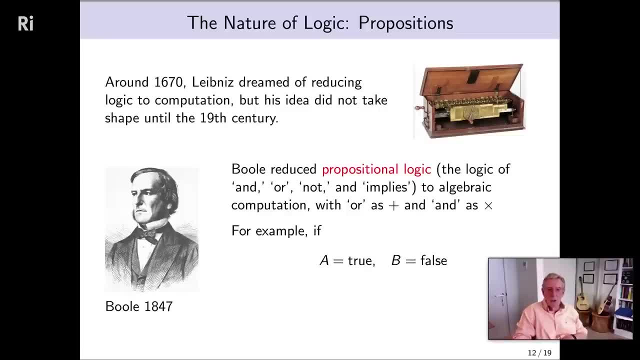 so let me give you an example. suppose we have propositions we call a and b and a happens to be true and b happens to be false. in that case a plus b, which is a or b, is also true, but a times b, which is a and b, is false. so very simple computation and you can elaborate. 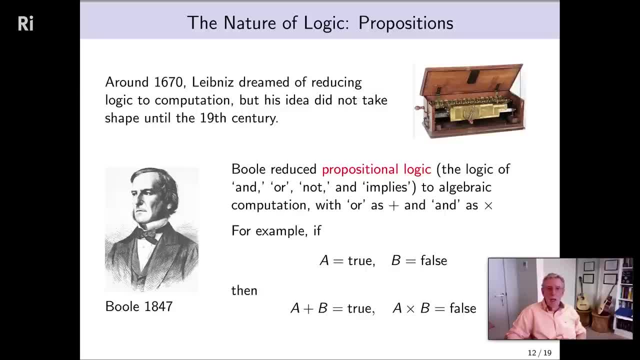 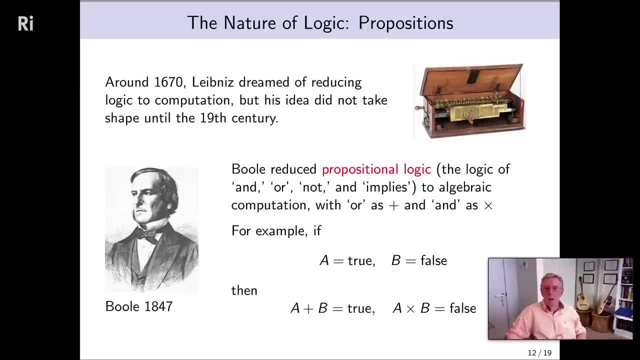 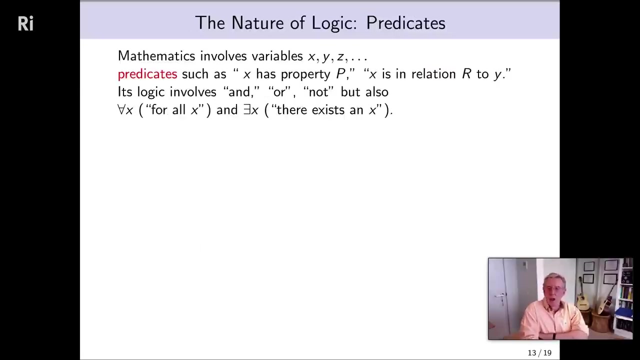 um, given truth, values of the variables, abc, etc. you can calculate by these rules, simple arithmetic kind of rules, what the value of the proposition is, whether it is true or false. uh it, it corresponds, corresponds rather beautifully to arithmetic addition and multiplication, But unfortunately it's not a rich enough logic to describe mathematics. because if 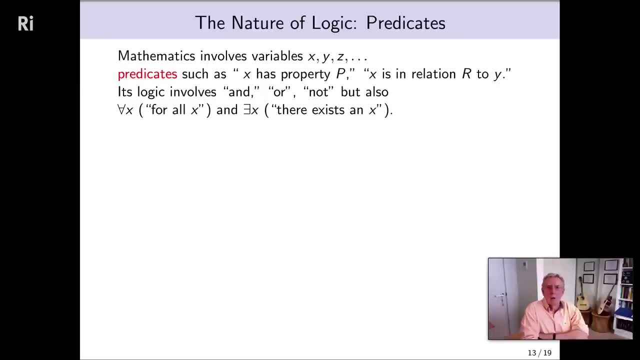 you think about mathematics. mathematics involves variables, x, y, z and so on, which could stand for numbers or points or lines or sets. many different things, many different interpretations of the variables are possible. And then there are predicates, such as properties or relations. 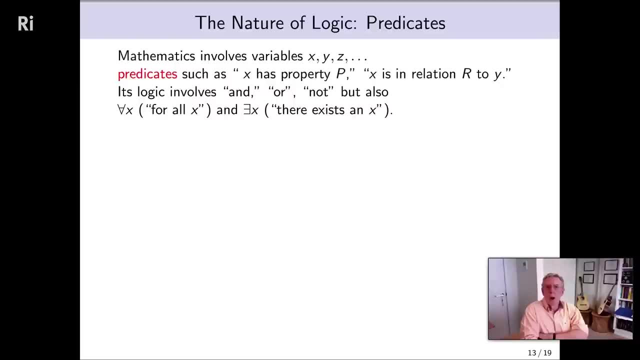 So you can say things like x has property p, or x is in relation r to y. So the kind of propositions in this logic are quite complicated And they require a lot of interpretation. you've got to interpret the variables, whether they stand for numbers or whatever. you've got to interpret the properties, whether property. 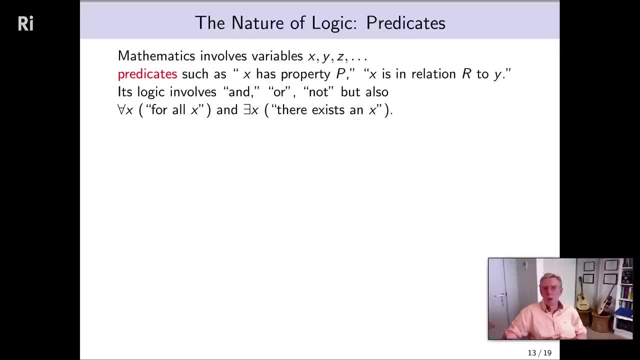 p is perhaps being even being odd. you've got to interpret the relations such as: maybe x is less than y or x equals y. All of that has to be done before you think about combining propositions by end or not. And in addition to that, 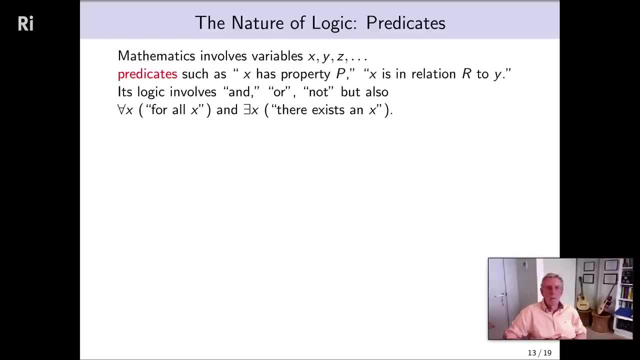 you've got to have quantifiers, as they're called, the for all x and there exists an x, And when you got all of that, then you can. you can state all the propositions of mathematics. So this is the language strong enough to express mathematics. 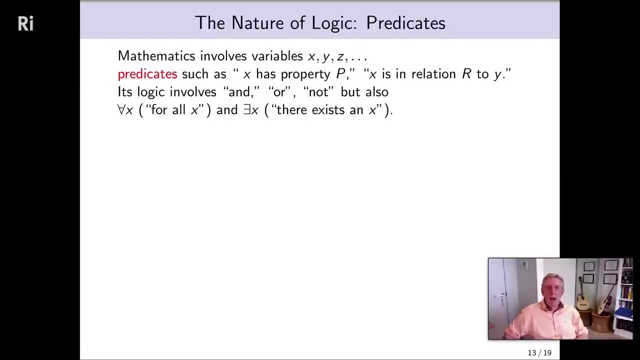 And it has logic ingredients. But how do you decide which are the logically valid statements, the statements that are valid under all possible interpretations? Now, an example of a valid statement would be say: if a has property p, then there exists an x, such that x has property p. 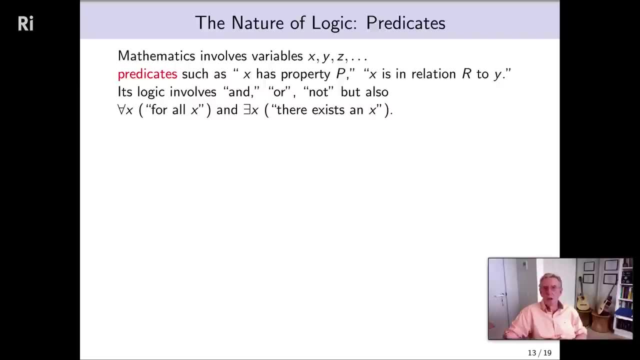 That's true for all interpretations of x and all interpretations of the property p. But how do you find all of those things? it's not simply a matter of calculating sums and products, like it is in propositional logic. Now, remarkably, the logic of the problem is that it's not always the same. 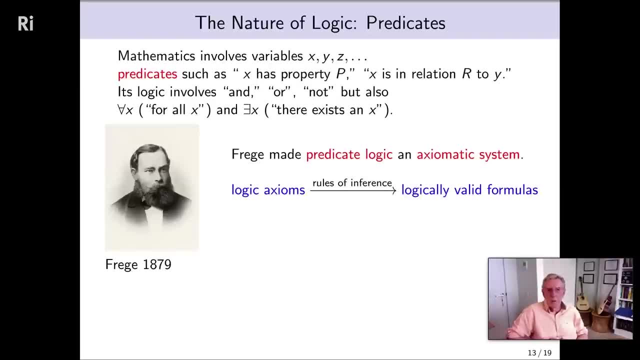 The problem is that it's not always the same. And what's interesting is that Brega- I think the German philosopher Brega- completely settled this question back in 1879.. He made predicate logic an axiomatic system. He found some logic, axioms which were self evident, self evidently valid statements. 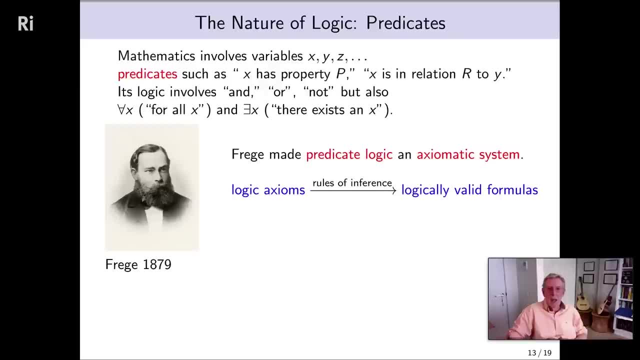 like the one I just mentioned about, exists an x, and he stated some rules of inference which enabled it, enabled you to derive new valid formulas from old ones, And he supposed- though he didn't prove- that his axioms and his rules 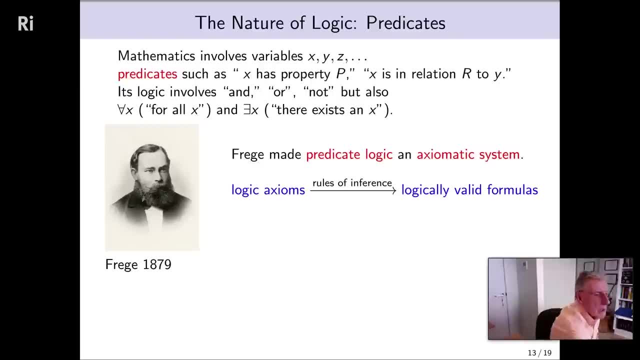 would give you all the logically valid formulas. Now, it wasn't known at the time whether his axioms and rules were complete in this sense. That was not known for another 50 years. But in fact it is true, Frege's axioms and rules are sufficient. 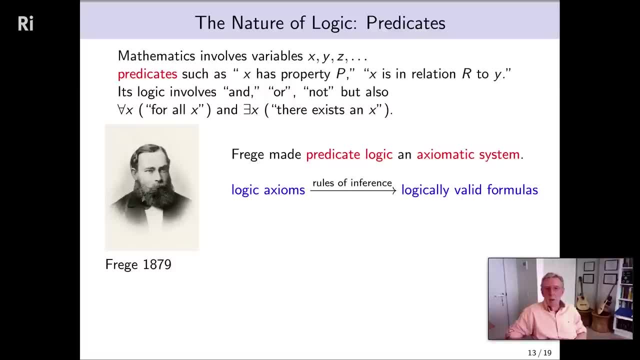 to derive all the logically valid formulas. And this gives a rather exciting possibility. Namely, you could describe an algorithm for generating all proofs and hence all logically valid formulas, And the algorithm would go something like this: You could list all the formulas with one-step proofs. 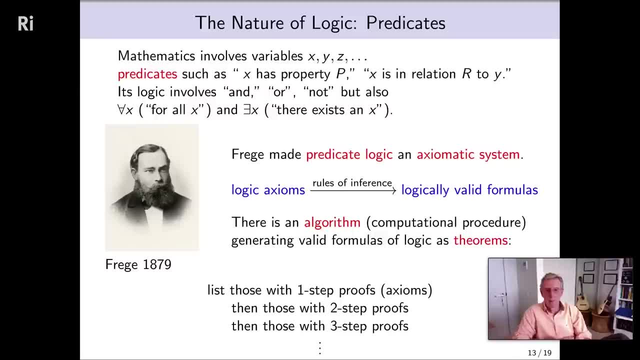 They're the axioms themselves. You simply write down an axiom and that's considered a proof of the axiom. Then you write down the ones with two-step proofs, the theorems that followed from the axioms, in one step. one application of a rule. 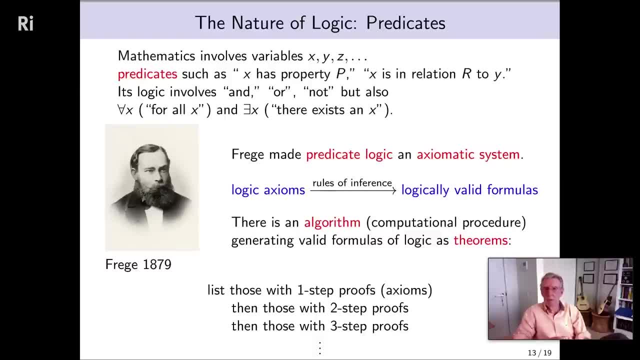 Then those with three-step proofs, those with four-step proofs, and so on, And so anything that has a proof will eventually be reached by this process. Now it's worth dwelling on this idea a bit. I should say that Frege didn't imagine this possibility. 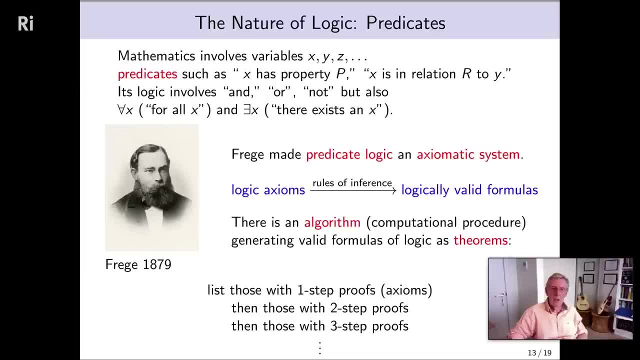 as far as we know, It was only seriously considered in the 1920s, when people began to think about it, When people began to think about calculations of this kind. And it's also important to realize what this does not do. It does not enable you to decide. 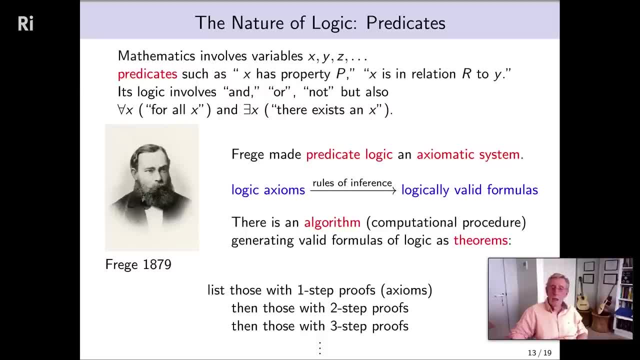 whether a proposition of logic is valid or not. If it is valid, you will eventually find it by this process, But you don't know how long you will have to wait. And if it's not valid, you may simply wait and wait in vain. 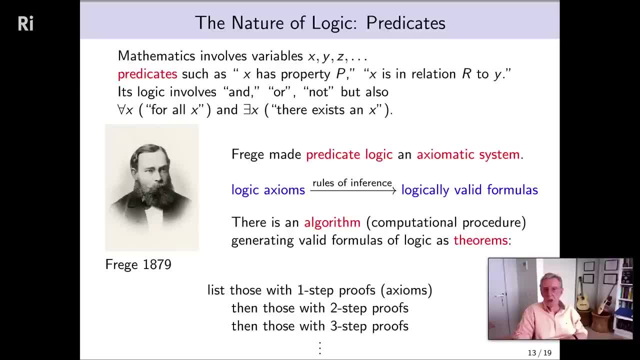 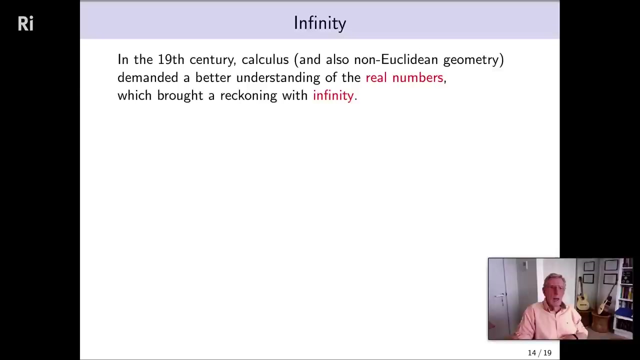 Forever, Because this process produces only valid proofs and not the invalid ones. So there is a slight catch to this. It's sort of one-sided: You can find all the valid formulas but not necessarily all the invalid ones. Now, this is an infinite computation. 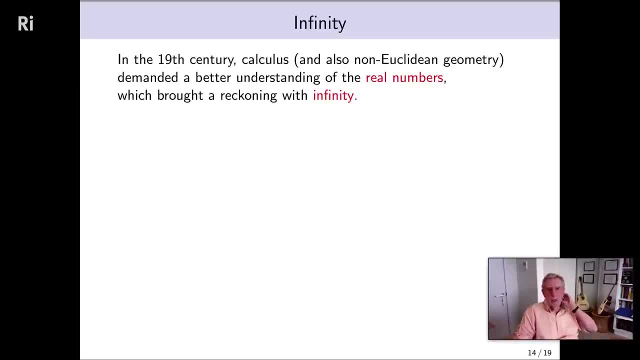 As I said, these things are quite reasonable but not considered valid Until the 1920s. But what then? in the 19th century, the concept of infinity was studied seriously for the first time, And the main reason for this was: 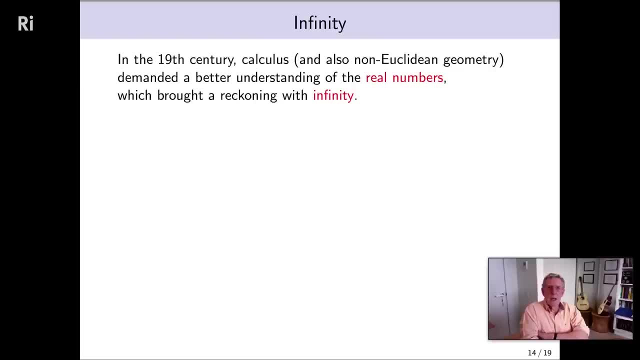 the need to understand the real numbers. Calculus, as we've seen, demands a better understanding of the real numbers. Another thing that happened in the 19th century was that non-Euclidean geometries were discovered. It was discovered that Euclid is not the only possible geometry. 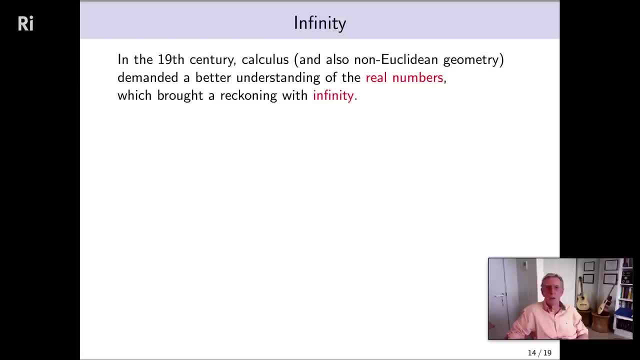 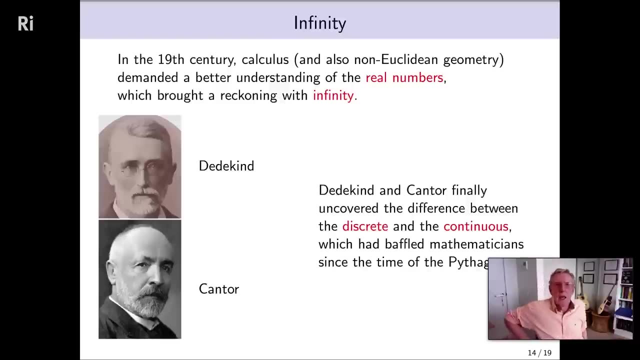 And so a common foundation for all geometries was needed, And the real numbers seemed the best way to get there. But to understand the real numbers you've got to understand infinity, And the two mathematicians who contributed the most to this initial understanding were Dedicate and Cantor. 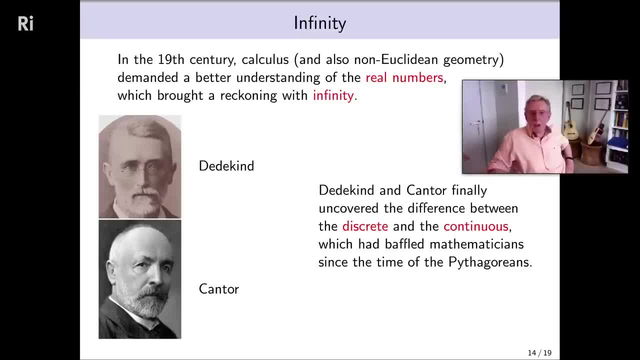 Between them, they uncovered the difference between the discrete, which is exemplified by the natural numbers, and the continuous, which is exemplified by the real numbers, And which had been a thorn in the side of mathematicians really since the time of the Pythagoreans. 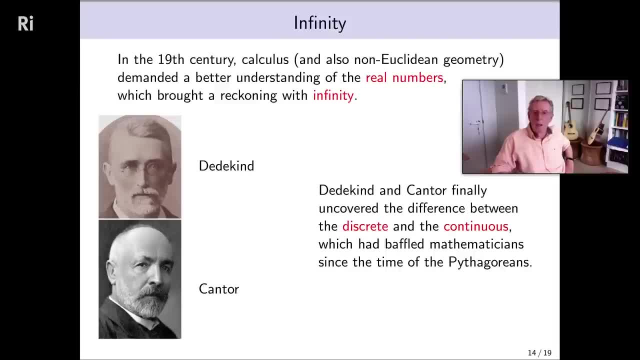 The first problem about the discrete and continuous was really the discovery that root two is irrational. The continuous real numbers did not match up to the real numbers. They were just the discrete natural numbers in some sense, But the Pythagoreans didn't really. 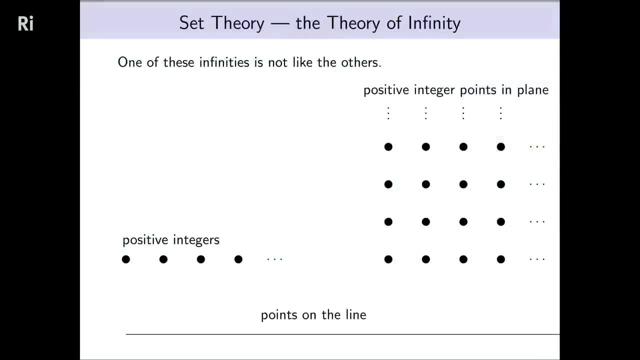 couldn't really put their finger on what the difference was. Now let me illustrate the difference first with a picture. The positive integers and what I've called the integer points in the plane are examples of discrete infinities. They're certainly infinite. 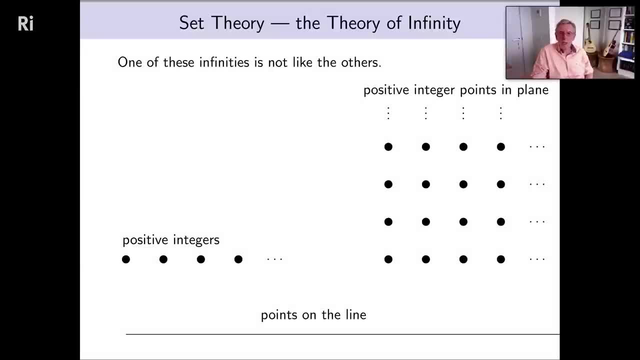 but you can see, their individual members are distinct and separate from all the others, Whereas the points on the line, somehow difficult to separate, They all hang together somehow. Now another way to pinpoint the difference between these two infinities. 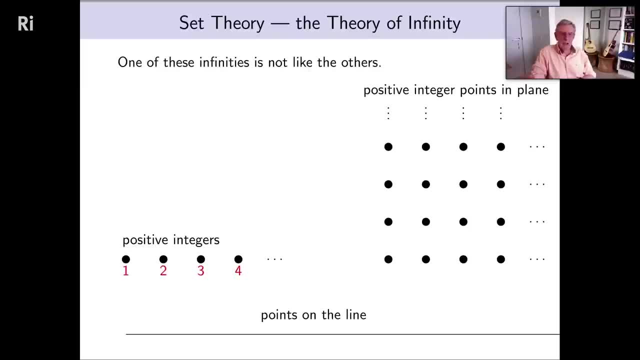 is to think about counting them, The positive integers. of course. you can count one, two, three, four. You can say: there's a first one, there's a second one, there's a third one, a fourth one, and so on. 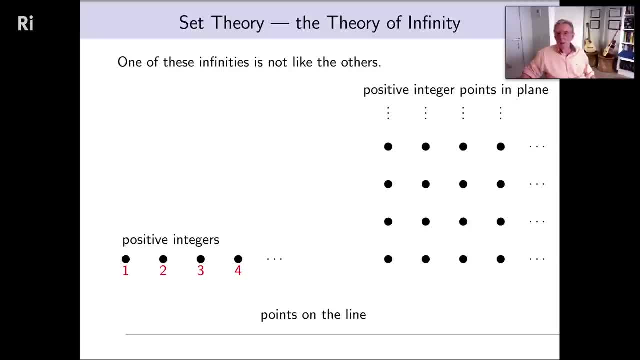 The same is true for the integer points in the plane, Not quite so obvious, but you can count them by, starting at the bottom left-hand corner, number one, and then those next to it. nearest to it, number two and three, then nearest to those, four, five, six, seven, eight, nine, 10,. 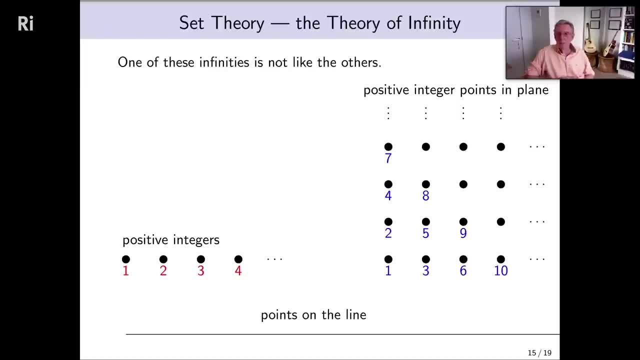 as I've listed there, And you can see that we, in this way, can give a number, a natural number, to every one of those points in the two-dimensional array. It's not at all clear that you could do that with points on the line. 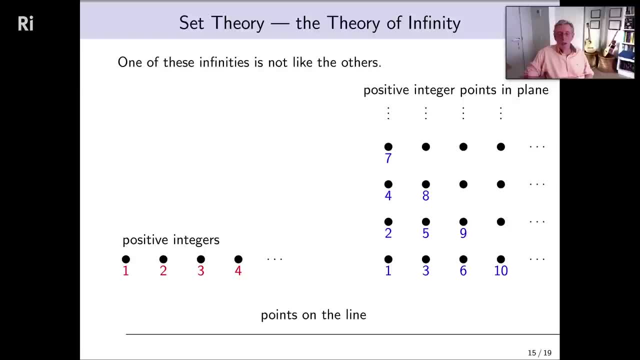 You might wanna say that the leftmost point is the first point, but there's no nearest point to the leftmost point. You've just gotta take a stab somewhere else for the second point And somewhere else again for the third point, And it's not at all clear that if you'll ever succeed, 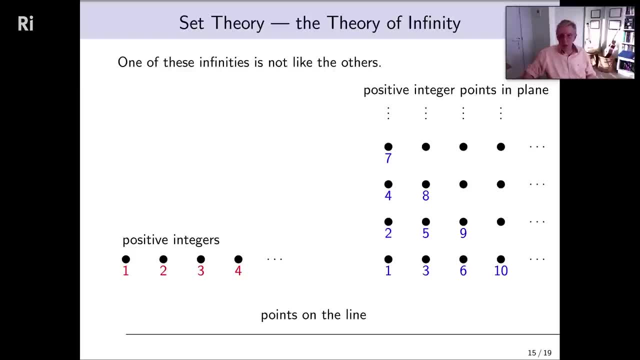 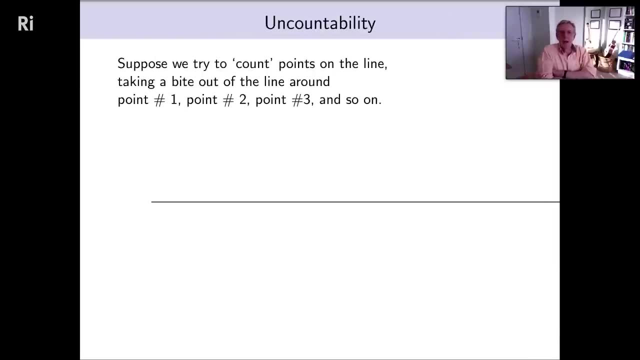 in giving integer numbers to all the points on the line. But let's try. let's imagine we find a way of counting the points on the line- Point number one, two, three and so on, And you won't see the points. 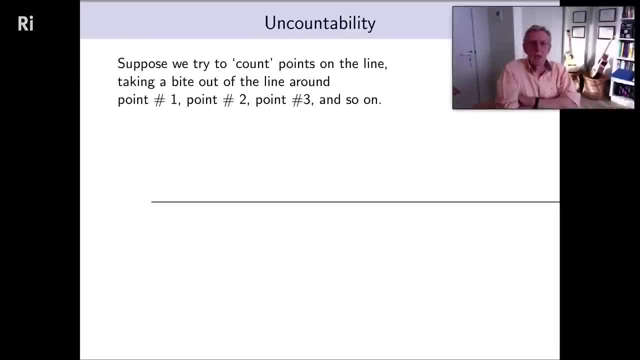 in the line. So I'm gonna take a whole byte out of the line around point number one and point number two and so on. So the point number one is in the middle of that disk. That's the first byte out of the line. 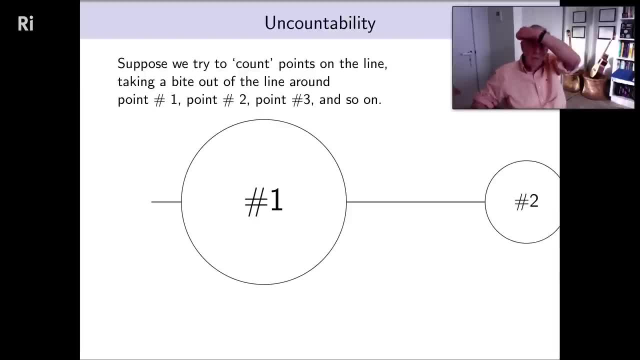 Point number two is in the middle of that one, which is a half as wide as the first byte. The third is half as wide as the second byte, and so on. I keep taking bytes around the points I'm enumerating, each time half the size of the previous one. 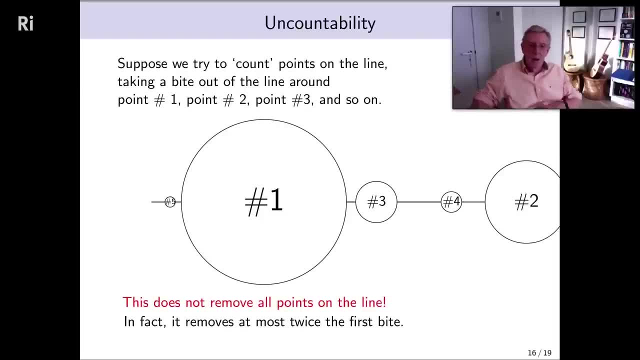 And I think you can see where I'm going with this. I'm not gonna remove all points. I cannot possibly remove all points from the line in this case, because I've removed at most twice the first byte, As I'm sure you know: a half plus a quarter. 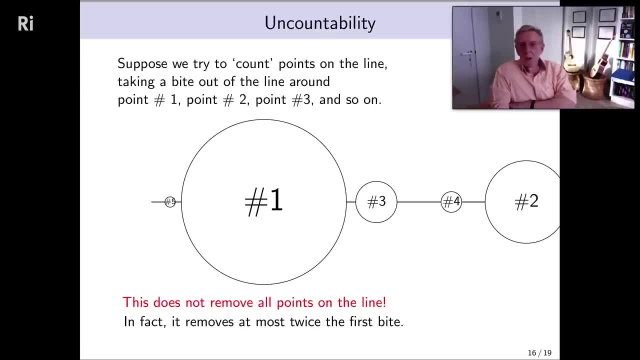 plus an eighth, plus a 16th, et cetera. I only used up the first byte, So I've got a finite amount of the line. We must have missed most of it in trying to enumerate points Now. I like to think that Euclid or Archimedes could have thought of this because they were well aware that you could add up an infinite number of pieces and get a finite object. For instance, Euclid found the volume of the tetrahedron by forming a line, And Archimedes found the volume of a parabolic segment. 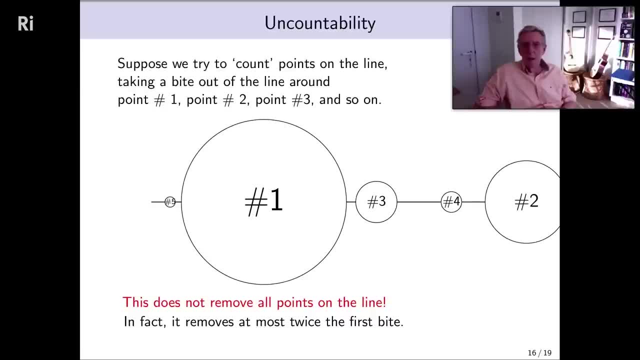 which is a finite slice off a parabola, by adding up infinitely many triangles. They were well aware, indeed, of the infinite geometric series which is involved here, So they could have done this, but as far as we know, they didn't. 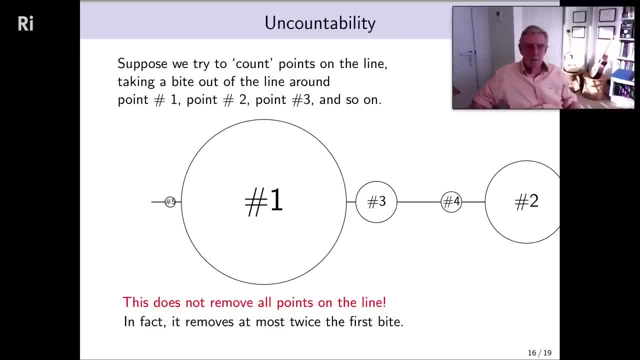 And indeed you may be a little worried about the fact that you can't get a whole lot of this in a single line, but you can get a whole lot of this. So I'm worried about this argument because I've not shown you any specific point. 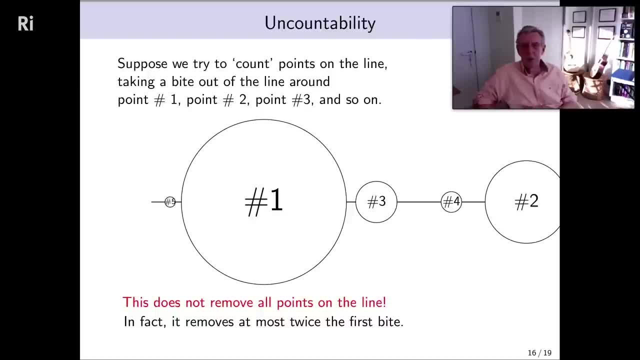 on the line that I've missed. I've shown that there must be many points that are missed in this process, but I've not pointed to even one of them, So you could doubt the processing on those grounds. So let me show you another way. 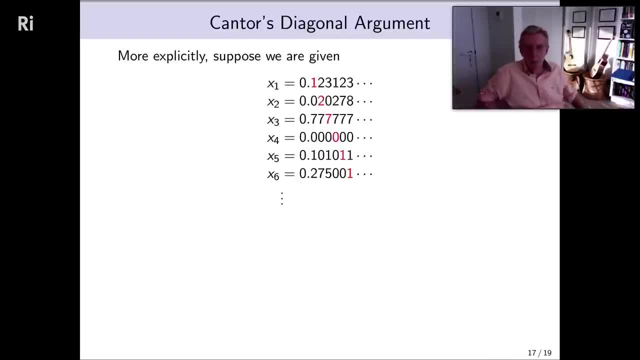 which is more explicit and really finds the missing point. As we know, the numbers on the line are the same as real numbers, and real numbers can be given by infinite decimal expansions. So I've taken a hypothetical infinite sequence of points X1,, X2,, X3,, X4, et cetera. 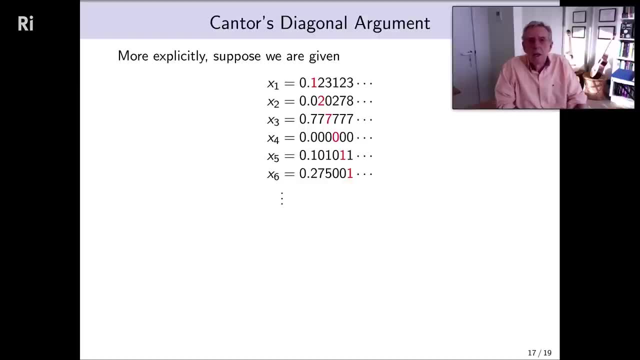 and described each of them as an infinite decimal expansion. And the actual expansions do not matter at all. but just for the sake of argument I've written some particular numbers here And I've highlighted the first digit in the first number. second digit in the second number. 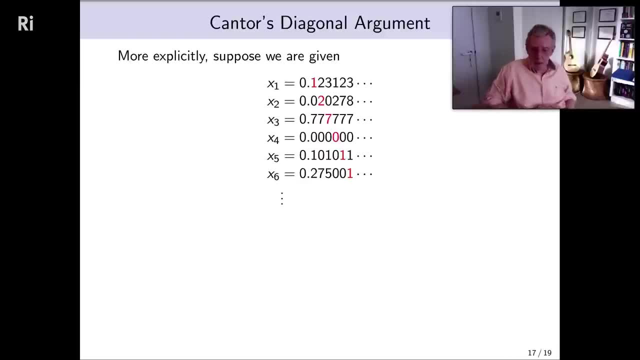 third digit in the third and so forth in red. And you see, when I've done that, I can write down a number which differs from all of the infinitely many numbers on the list, And the rule for making this number is very simple. 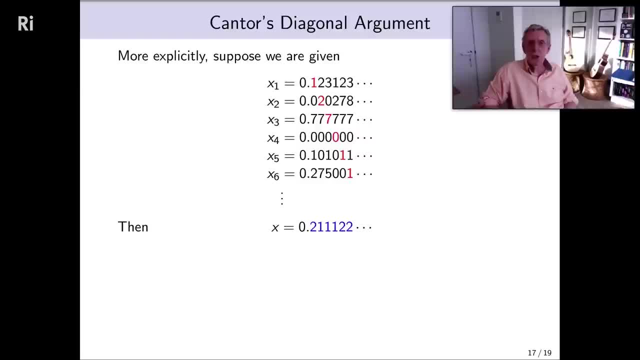 If there's a red one, you change it to a two, as I've done in the first decimal place. If the red number is not a one, you change it to a one, which I've done for the other places. So I've made a number here deliberately different. 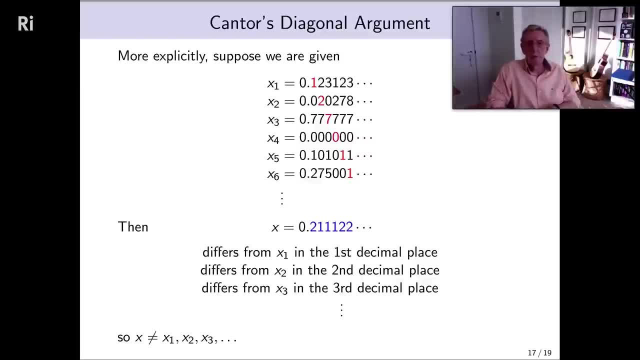 from each of the numbers on the list. It differs from X1 in the first decimal place, X2 in the second decimal place, X3 in the third decimal place. So the beauty of the diagonal argument, as this is called, is that you've got an infinite number. 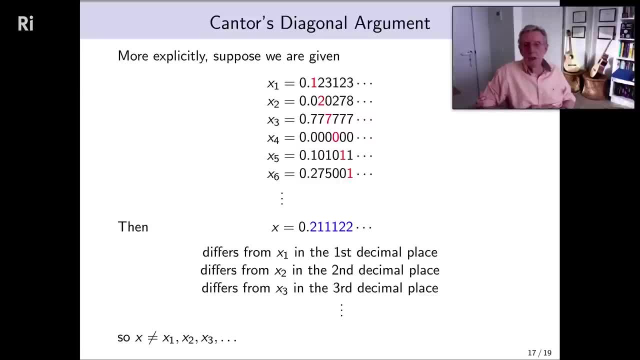 is that you've got an infinite amount of room to make this new number different from all the infinitely many other numbers. So this X that I've made and computed very explicitly is different from all of X1,, X2,, X3, and so on. 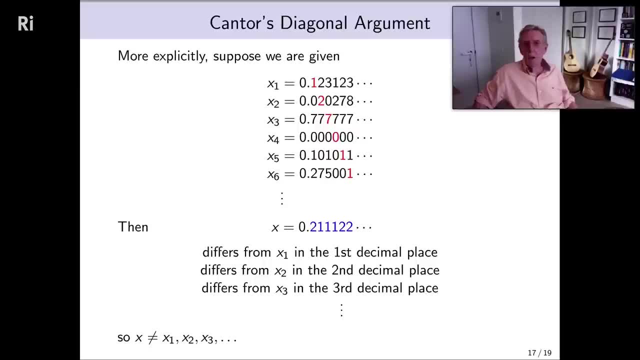 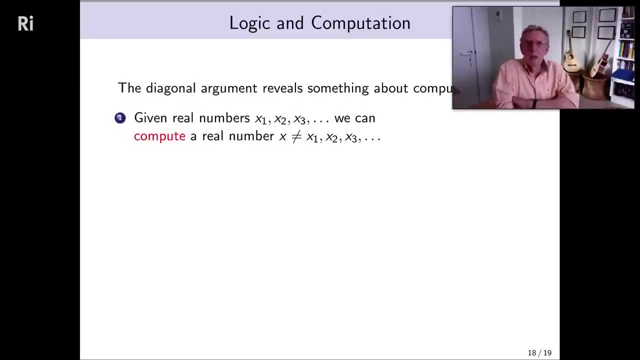 So suddenly the idea of computation has come into the story. The diagonal argument reveals reveals something very interesting about computation. It shows that given real numbers- X1,, X2, X3, infinitely many- we can compute a real number different from all of them. 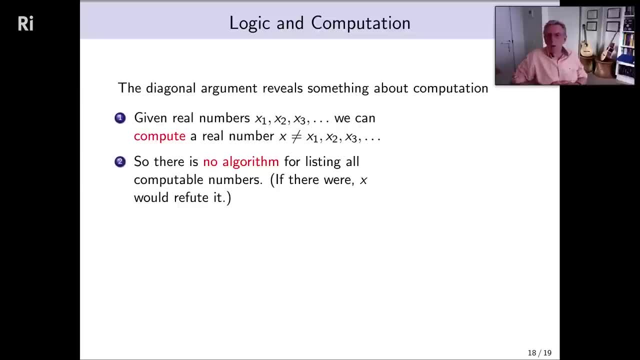 It follows that there's no algorithm for listing all the computable numbers, because if there were, we could do it, and then X would refute this algorithm by making a new computedom number. It follows, in turn, that there can be no algorithm for looking at algorithms. 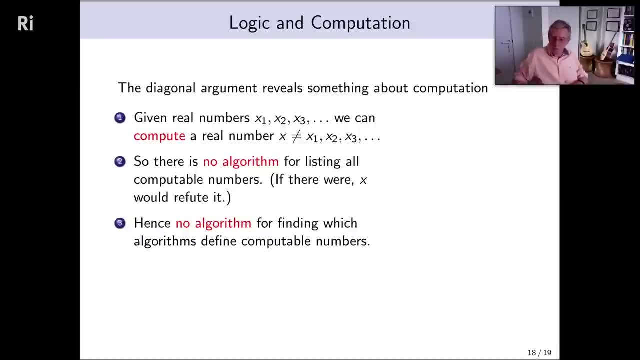 and finding the ones that define computable numbers. Algorithms are just something you could write down, say in some programming language, So you could list all the algorithms, certainly, but you couldn't pick out the ones that define computer numbers. So this tells us something about compute numbers. now, 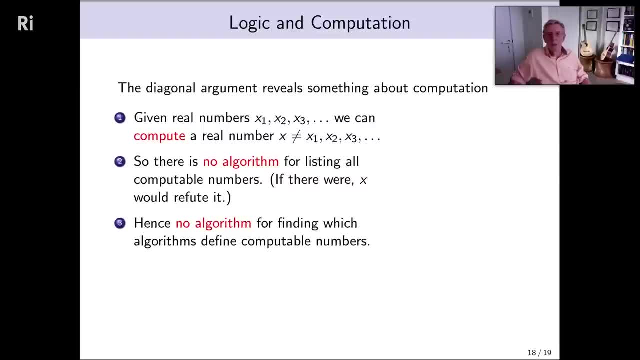 about non-existence of algorithms for certain problems. also, it tells us something about axiom systems, because axioms produce true statements, and if you suppose there was an axiom system for generating facts about computable numbers, it could tell you which algorithms define computable numbers, and we've just shown that that's impossible. therefore, no axiom system can produce. 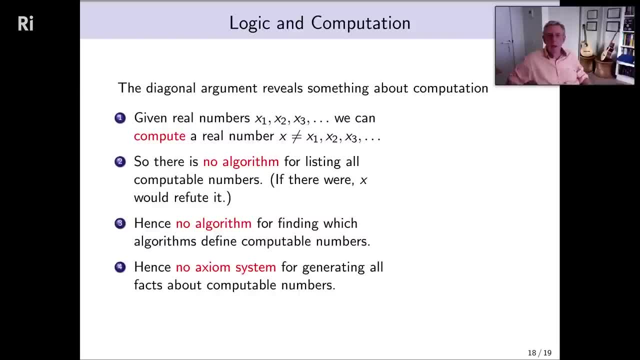 all the facts about computable numbers. now, what I've just described here are some baby versions of famous theorems in logic discovered by Post and Turing and Gödel. Post was the one who first thought about enumerating algorithms and realized that there would have to be unsolvable problems about 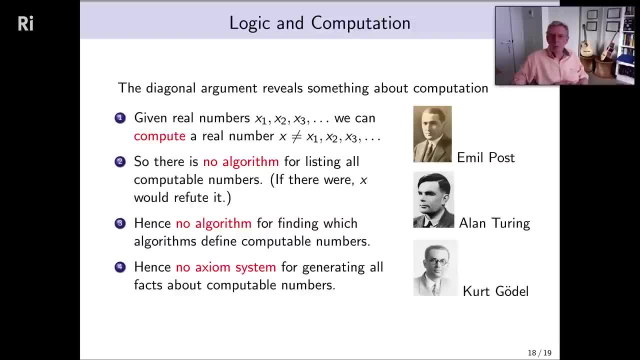 algorithms. Turing gave a specific definition of what an algorithm was in what's now known as the Turing machine, and he gave this exact argument about real computable numbers. in fact, his paper was called on computable numbers and Gödel was the one- independently of these two, incidentally- who found that no axiom system can generate all the facts. 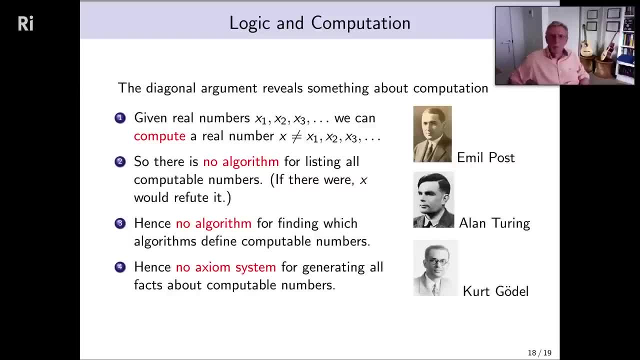 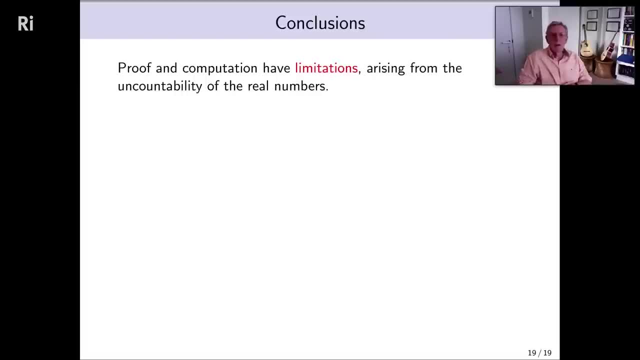 of mathematics. so, in conclusion, we've discovered, as a result of the diagonal argument, that proof and computation have limitations, and these arise ultimately from the uncountability of the real numbers. The limitations are that there are mathematical problems for which no algorithm gives all the correct answers. 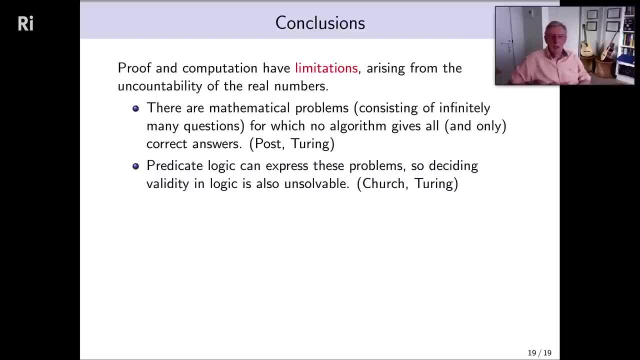 and it turns out that predicate logic, as I suggested before, can express all of mathematics, so it can express these problems and therefore deciding validity in logic is also unsolvable. Gödel showed that problems could be described in arithmetic in terms of just addition and multiplication, so there cannot be axioms to imply all the. 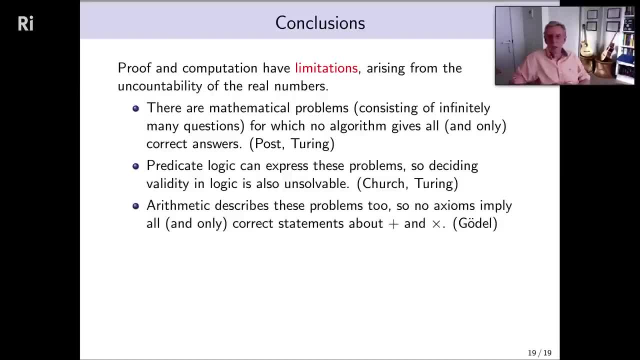 correct statements about addition and multiplication. as simple as that sounds, there's no axiom system to produce all the theorems. and to be a little more specific, if you consider polynomial equations now, polynomials are things you get from variables simply by addition and multiplication. and so if you write down an equation between two polynomials and ask: 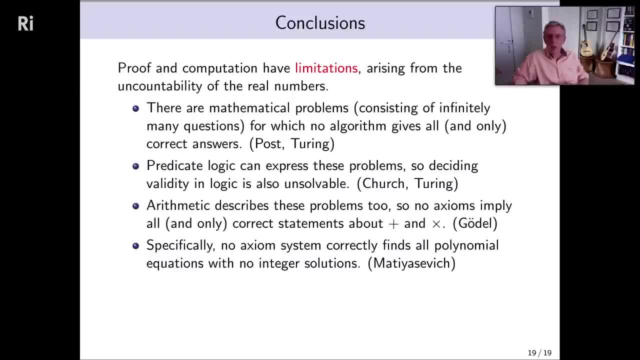 whether it has integer solutions. if the answer is no, you're not always going to be able to find that out. there's no algorithm for finding the ones that have no solutions. so, in the end, this diagonal argument has led it led us to very concrete limitations in in the power of logic in mathematics.